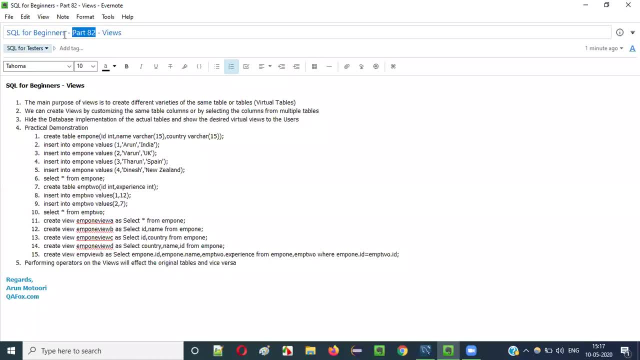 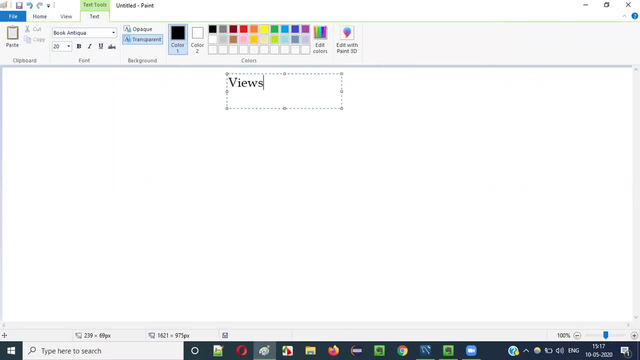 Hello everyone, Welcome to part 82 of SQL for Beginners series. In this video session I am going to explain and practically demonstrate on how to use views in SQL statements. So in this video session I am going to explain about the usage of views in SQL statements. 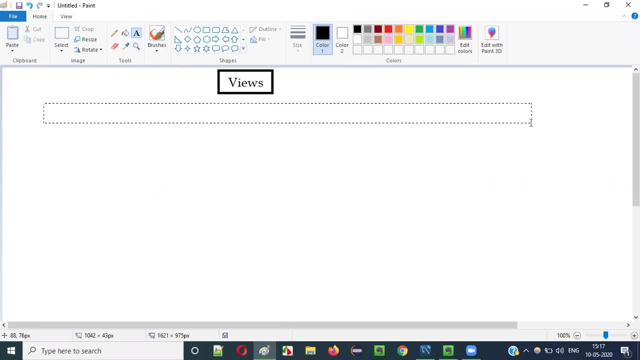 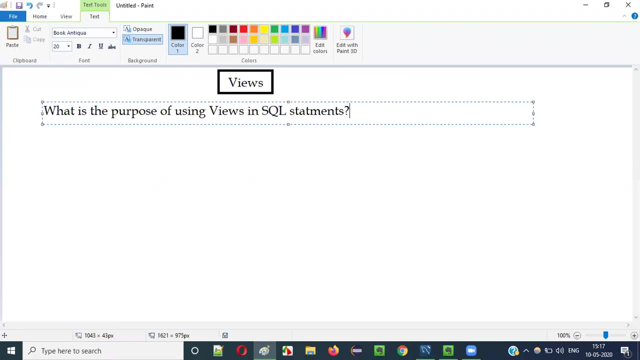 First, we need to understand what is the purpose of views, Views, What is the purpose of using views in SQL statements. We need to understand first. So what exactly are views and what is the purpose? You have to understand In order to understand the purpose of views. let me explain something. 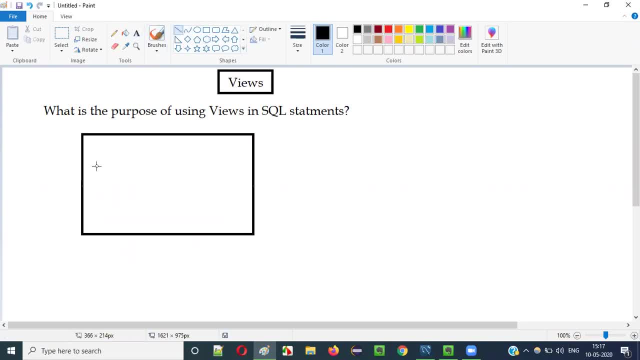 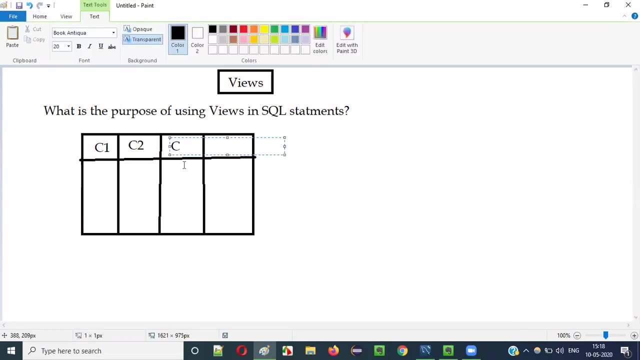 Let us say there is a table And it has some columns like this: Some four columns are there in the table And I am giving the column names as C1, C2. C3, C4. And let us say the table name is Table 1.. 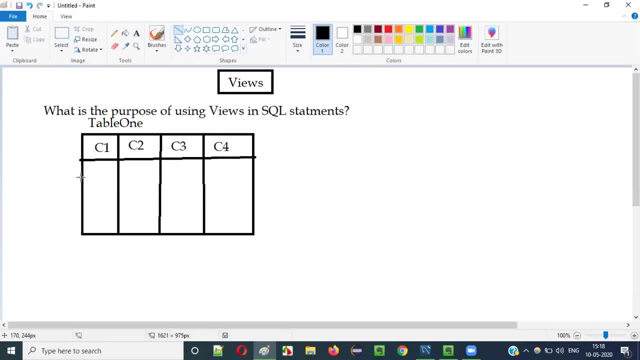 And it has some data Under the table. there are some records. There are some column records are there. Some data is there under all the four columns of this particular Table 1.. There are some data, That is, table records are there. That is fine. 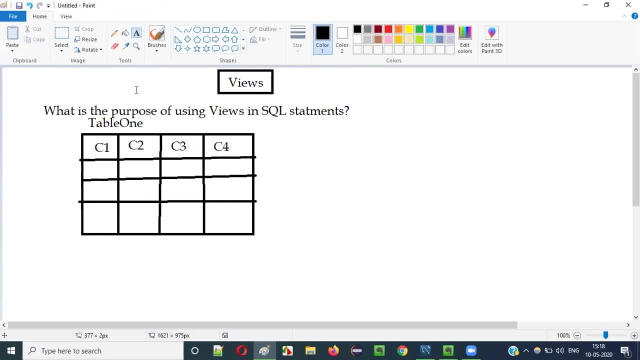 Now, tomorrow, what happened is we got a requirement where we do not want to display this entire table. We want to display this entire table on the web page And we wanted to have only first three columns. We do not want this fourth column. 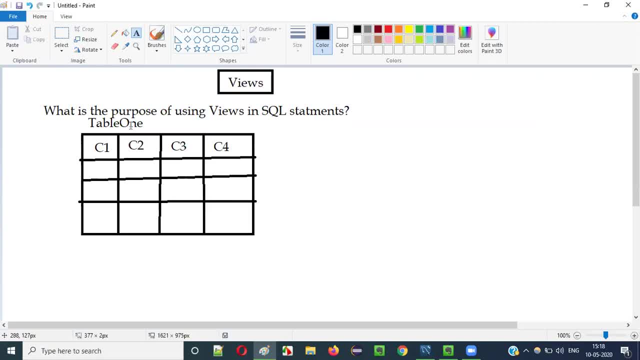 So another requirement came. So I cannot use this table, right, I cannot use this Table 1, because this Table 1 has C1, C2, C3, C4.. But only up to here, I want. I only want up to here. 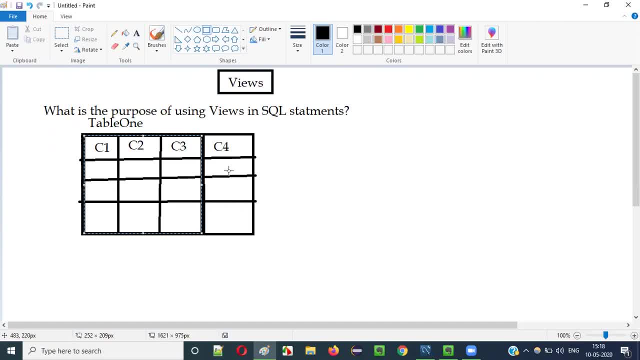 Without deleting this table or creating the table again. with this kind of thing, I cannot do right. Only these three columns are needed. What I will do tomorrow, what I will do, is I will create another table. Let us see, Let us say Table 2.. 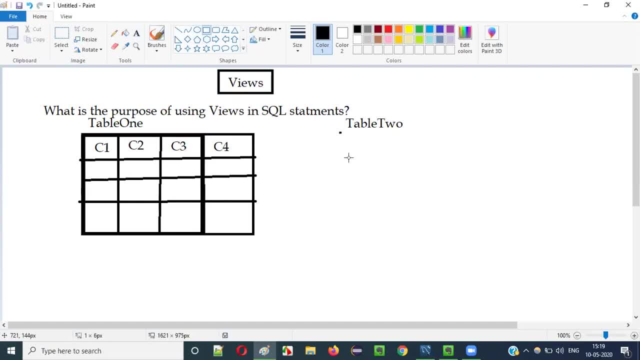 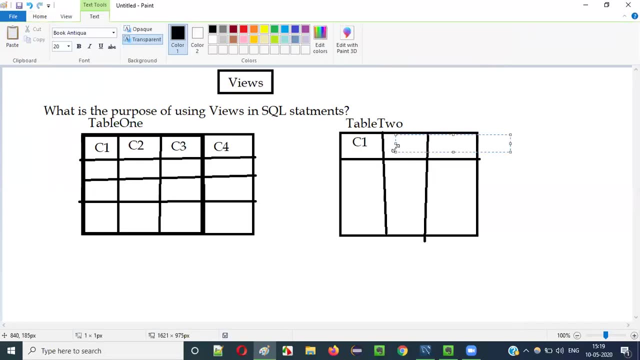 And this time I will create the table with only three columns, Only three columns, The required columns. So here it has only the first three columns, That is, C1, C2.. C1, C2 and C3.. 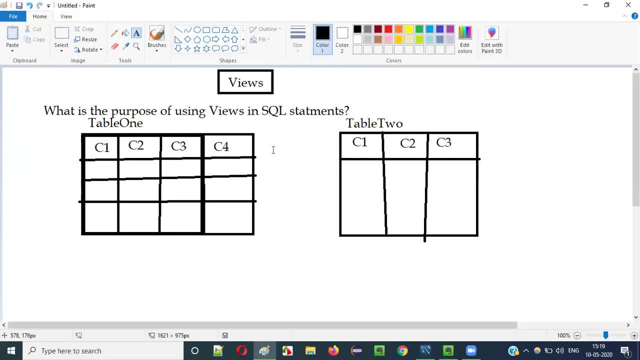 Again tomorrow. another requirement came, So here I have to create another table, Table 3.. It should have only C1, C3, C4. C2 column should not be there Like that. another requirement came. Again, another table we will create. 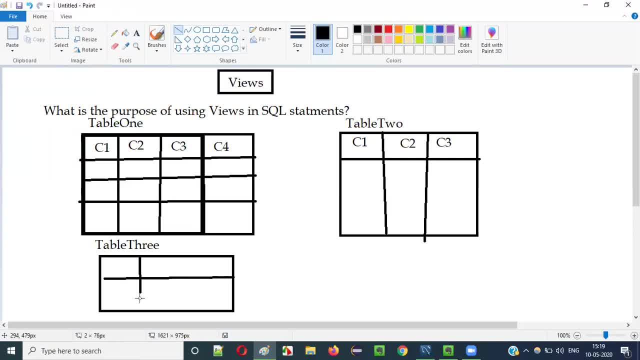 And it will only have again three columns. A different set of columns will be there here. The column names will be like C1, C3, C4. Like this. So, based on our requirements, we need to create two tables. 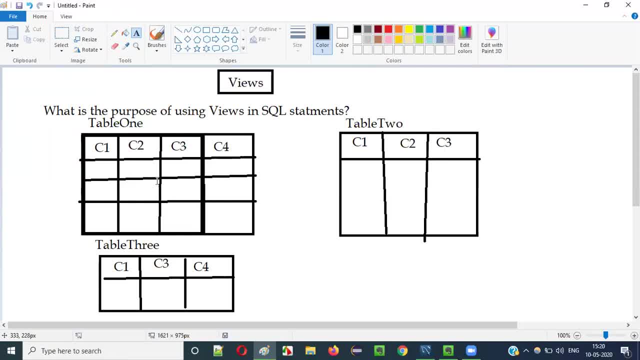 This is the same table. C1 is there in the main table, C2 is in this table, C3 is in this table. All these things, all the new table columns, are already there in this first table, First table. But since there are small requirement changes. 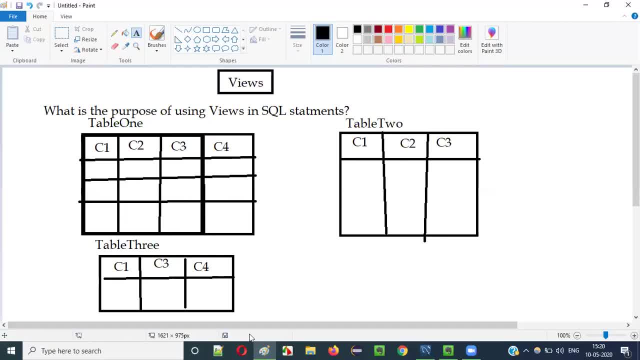 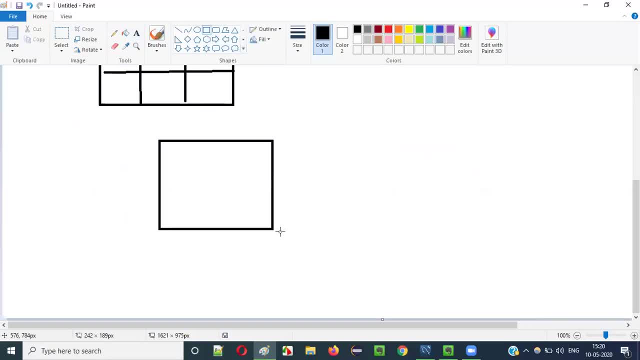 like: this column should not be there or this column should not be there. we have to create this kind of different table. That is the problem. And one more situation will come there: We have two tables. So this example is done, guys. 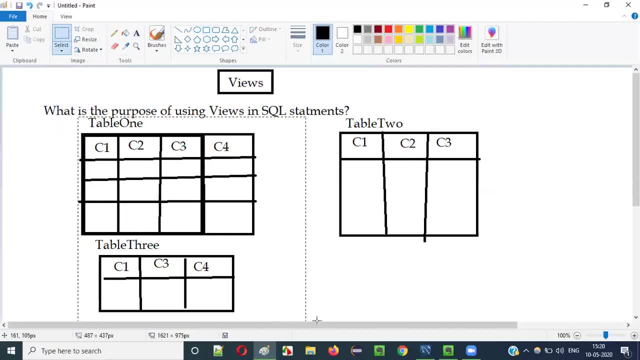 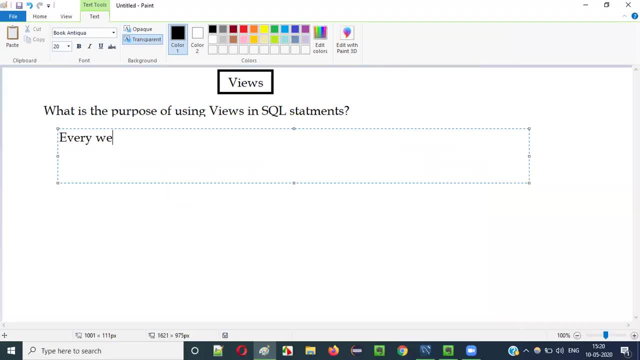 Why we need views. Because every time we need a small change in the existing table, we need to create a separate table. Let me write down here: Every time we need a small change in the existing table, what we have to do. We need to create a new table. 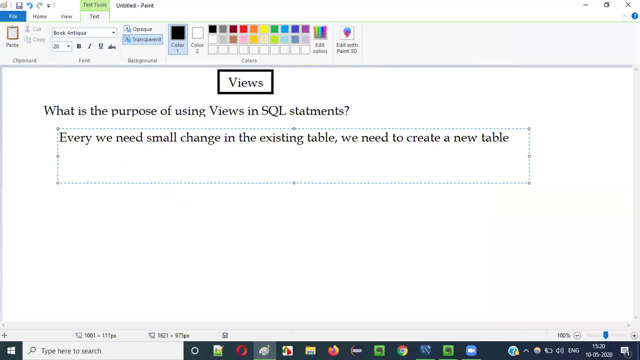 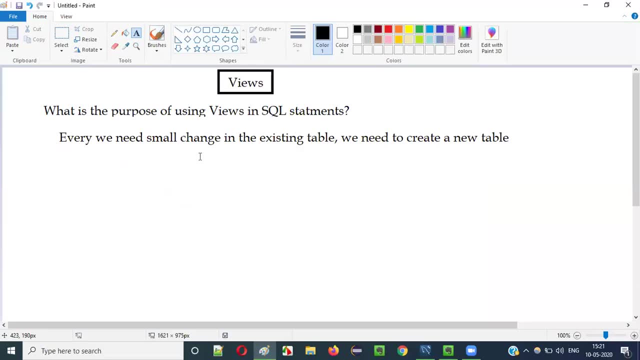 For every small change, that column should not be there. for every new change we have to create another table. So do we have to create like that? Not required, Because all the columns are there in the main table. Original table. 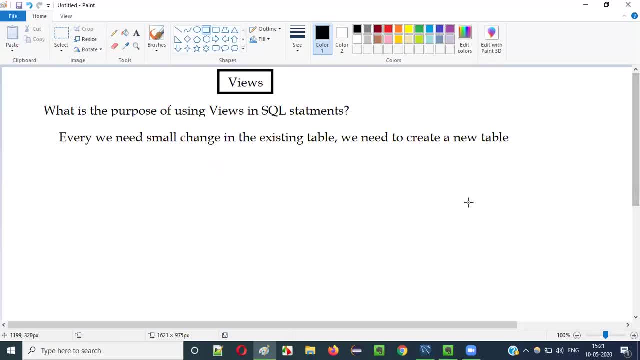 All the columns are there in the first table. Why should I create more tables just for the small changes like fourth column should not be there. second column should not be there in the resultant table. There should be some solution. The solution is nothing but views, guys. 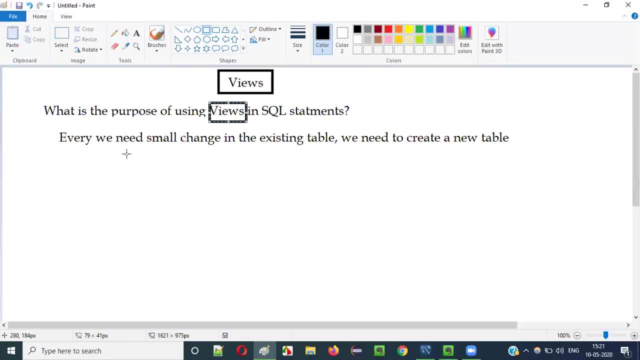 I will explain later point of time. I will explain how to use views. For now, understand the requirement why we have to use views in the SQL statements First, just for the small changes in the table. we don't have to create multiple tables. 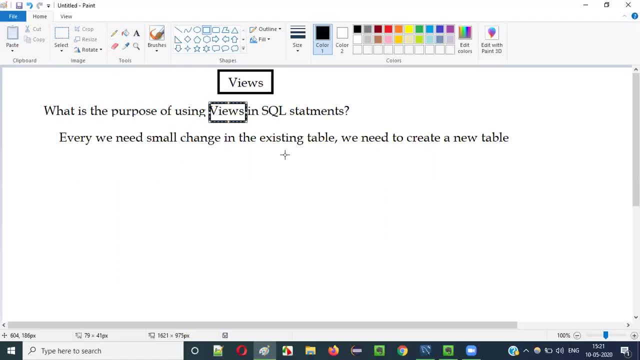 For different categories or types of the tables. we don't have to create multiple tables Just because of the smaller changes in the number of columns and all those stuff. There is a solution for that. That is nothing but views. Another place where we need views are 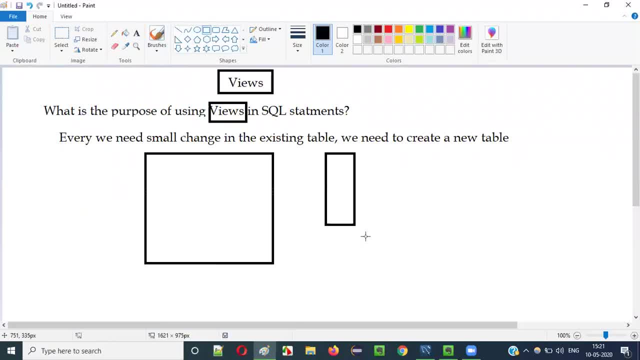 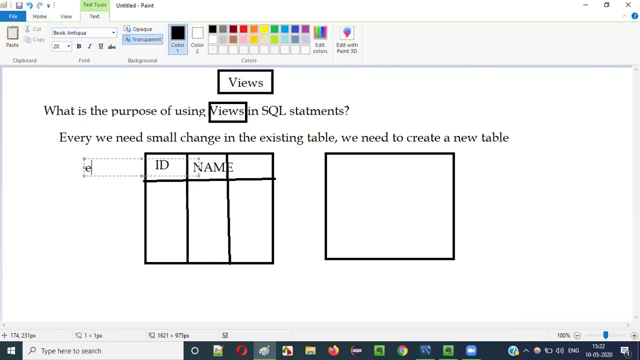 let's say there is two tables. There are two tables. In one of the tables there are three columns like this: The first column has a name as ID Here name Let's say this is an employee table. Let's call this EMP1 table. 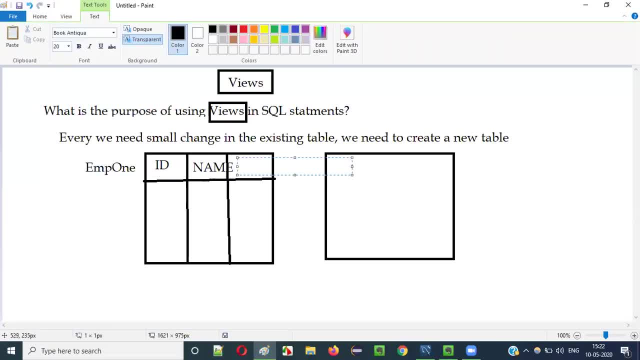 This is an EMP1 table. Here columns are ID, name, experience, And there is another table which has like this kind of columns. Again, here also we have ID, And here we have country And city, Country, city- This is also an employee table. 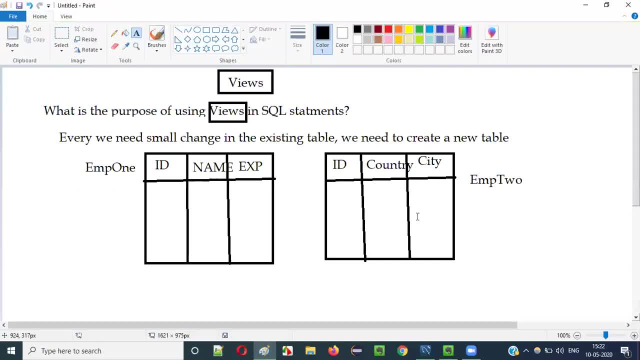 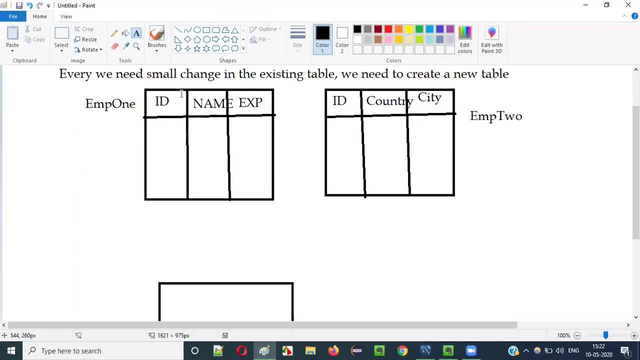 But a different employee table, EMP2 table. In the first employee table we have ID name, experience columns And in the second employee table we have ID, country, city. But what happened is tomorrow you got a requirement where you need a table In such a way that it has: 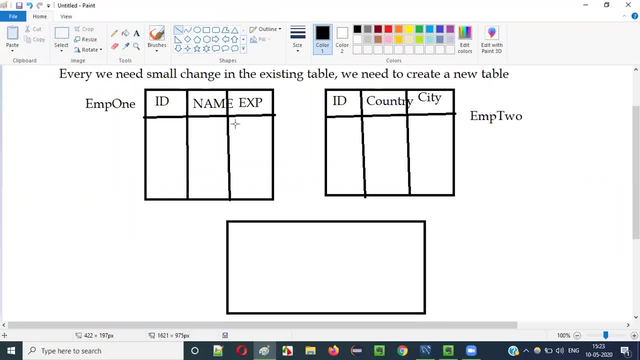 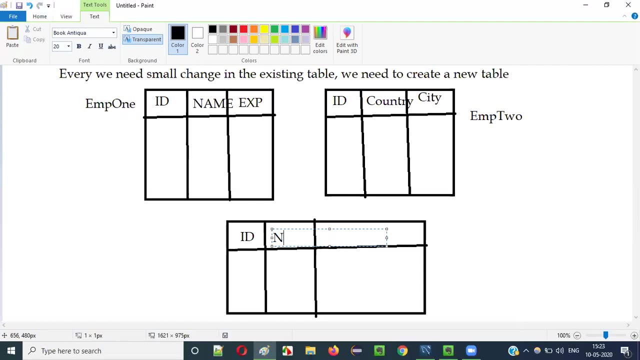 this type of columns, It should have this columns, That is, it should have ID, It should have name, Then it should have experience, It should have country, It should have country And it should have city, Country and city. Like this I want. 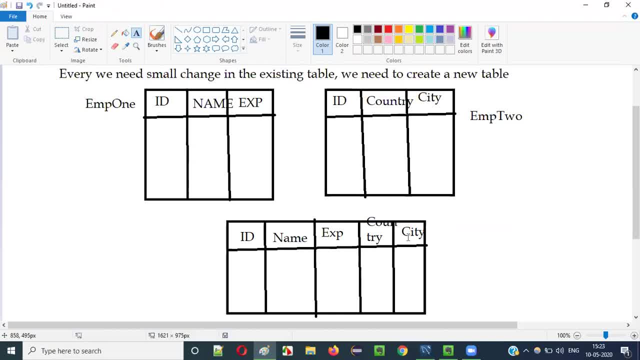 another table. The requirement came where we need to create a table, something like this: But in the database already there are two tables. Two different tables are there. One table already has ID name experience that this required table has, And another table has ID country city. 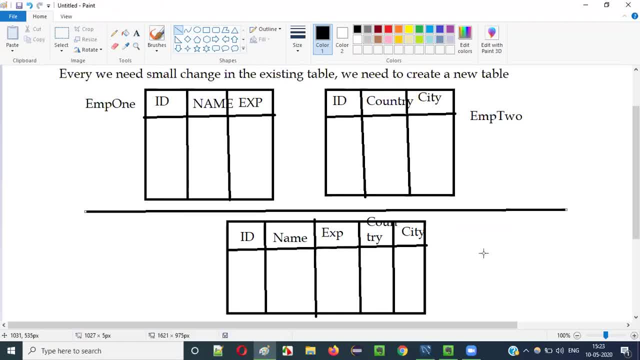 Now how to get this table. I have to create another table. I may have to create another table, like EMP3 in real time, But why do we have to create more number of tables? Already we have all the required columns and data in the. 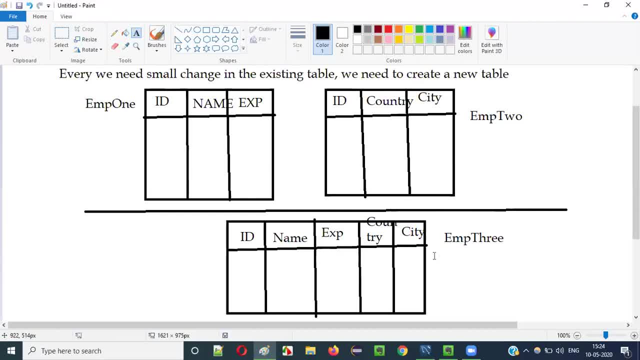 existing tables in the database. Again, just because of this kind of requirement, where we need all this different number of columns that are there in both the tables, Why we have to create another table. To overcome this problem, we have to use views. again, We have to use views. 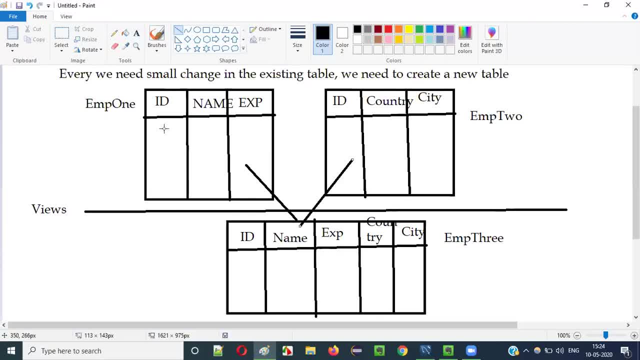 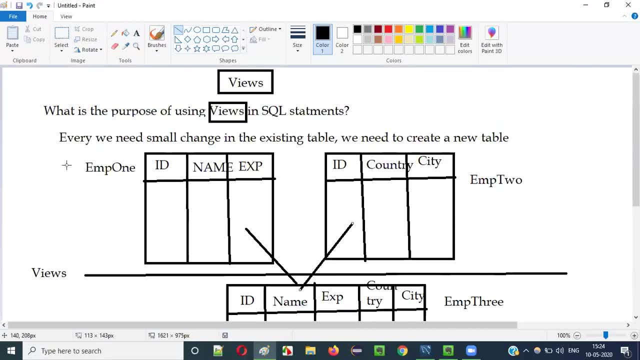 So, using views, what we can do is we can get the records from both these tables And we don't have to create the solution. So for every small change in the existing table or tables, we need to create a new table- This thing to overcome this kind of problem. 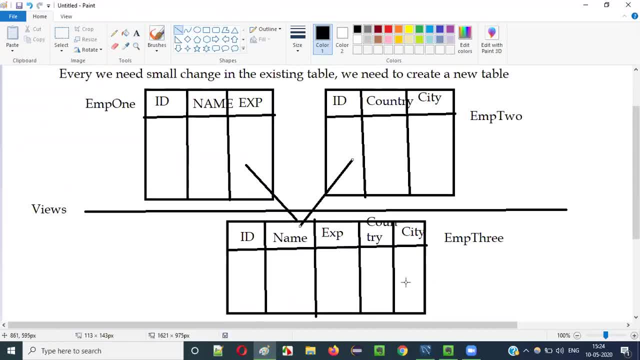 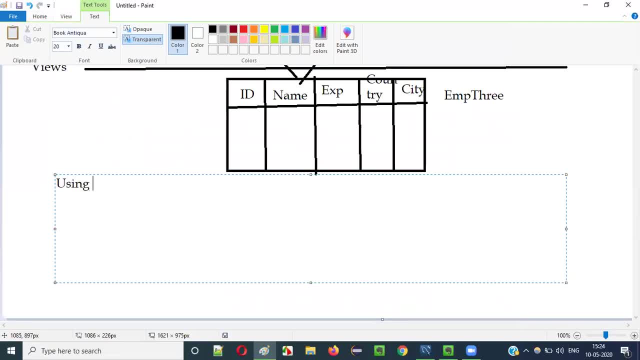 we need to go for views. Using views, we don't have to create new tables unnecessarily. So what is the purpose of views? Now tell me. To conclude: using views, we can overcome the need for the need for creating more tables. Creating more tables. 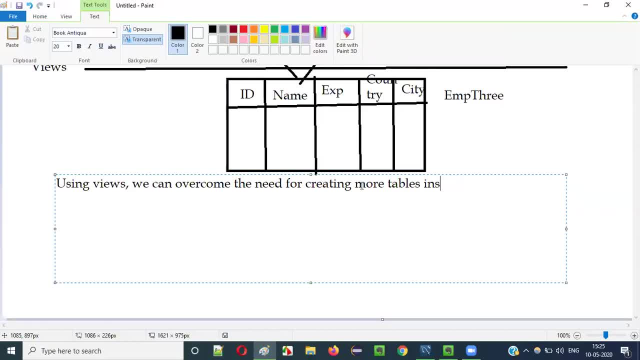 Instead of using views, we can overcome the need for creating more tables, even though, even though the required columns and data are available in the existing tables, Even though the required things are there in the existing table, but just to get that 5 columns or less, number of columns or more. 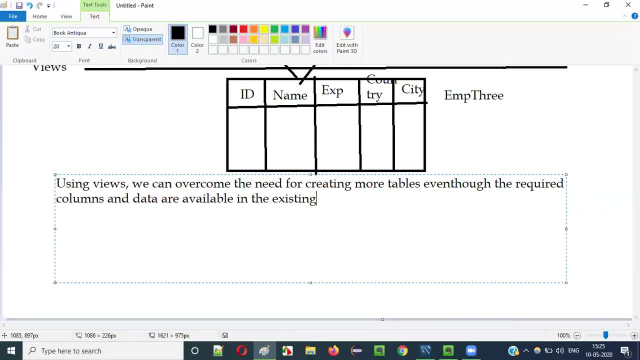 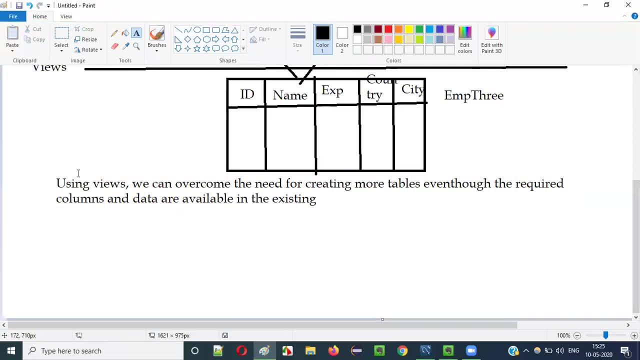 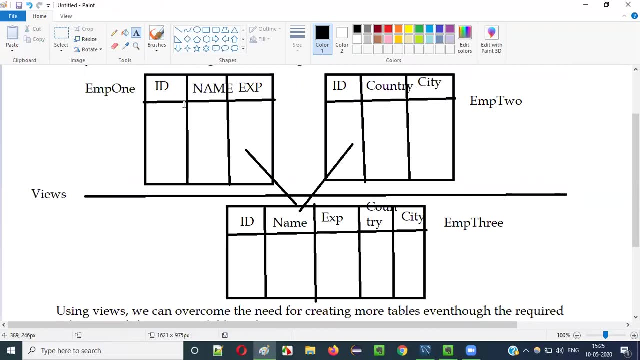 number of columns from different tables or from the same table. we need to create multiple tables In order to overcome this. we have to use views. We have to use views. What views will do? what views will do is like they will create a replica, kind of replica kind of thing like, for example, 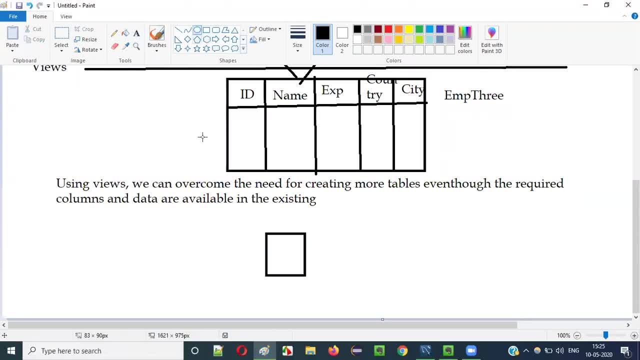 you are the person. let's say: you are the person, this is you, and there is a mirror before you. So when you stand before the mirror, what will happen? The same copy of you will be displayed in the mirror. So views are something like this, guys. 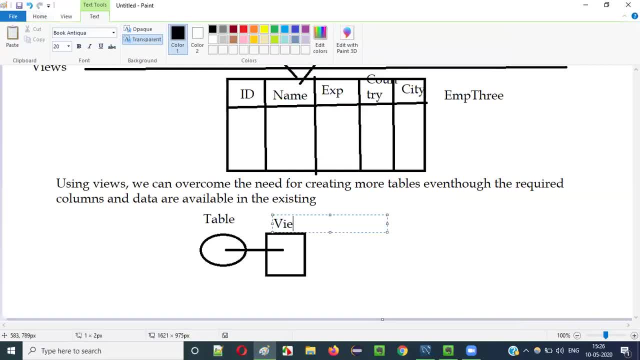 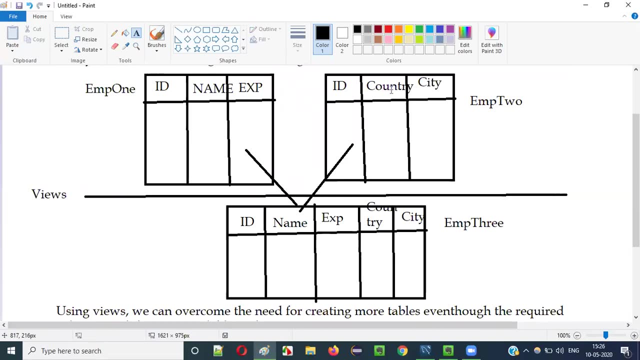 This is a table and using views we can create a mirror image In whatever the way you want to see. There are some different type of mirrors which have extra capabilities like that. So these mirror views are like: you can display different columns from different tables into a single table. 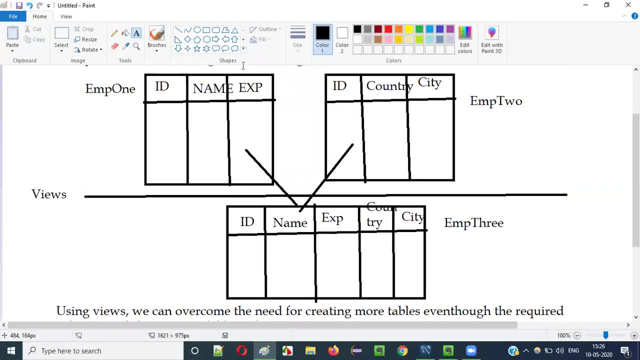 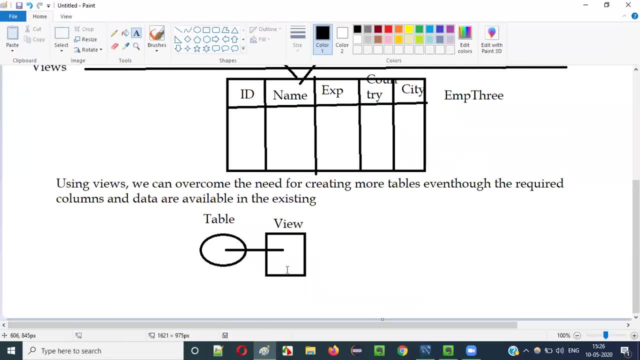 kind of thing That is also possible. Or if you have a single table and in that instead of these 3 columns you want only id and name, That also can be displayed with the help of views. It is a magic kind of mirror, guys. 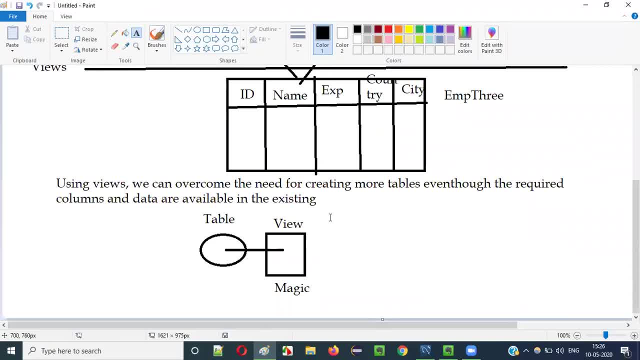 Not a straight forward mirror. It is a magic kind of mirror where, even though you are thin, you can look fat, or even though you are fat, you can look thin, Something like this. So, even though this particular table has 3 columns in the mirror, you can display 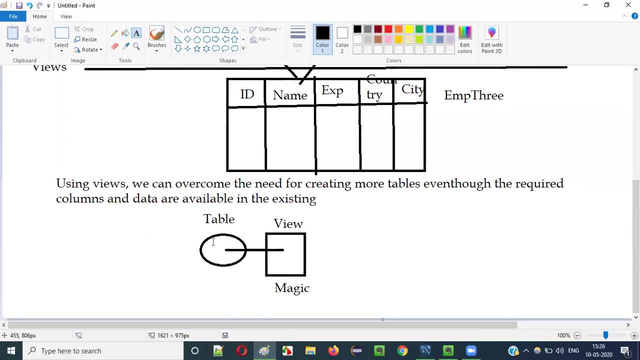 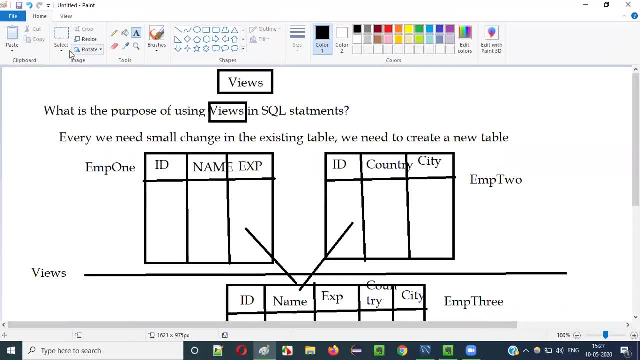 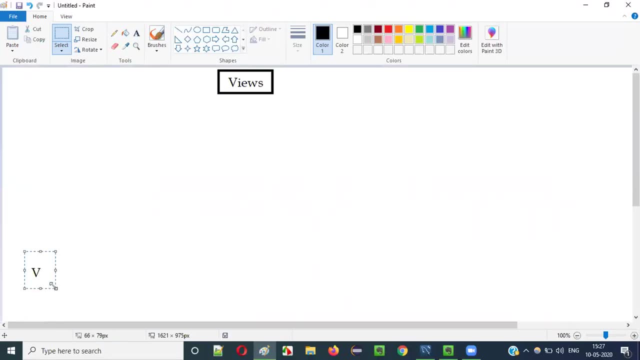 2 columns, or as it is also possible As it is, whatever you are, As it is, if you want to get displayed, also is possible. So again, again, if I have to explain about views, If I have to explain about views in a different way, Views are nothing. 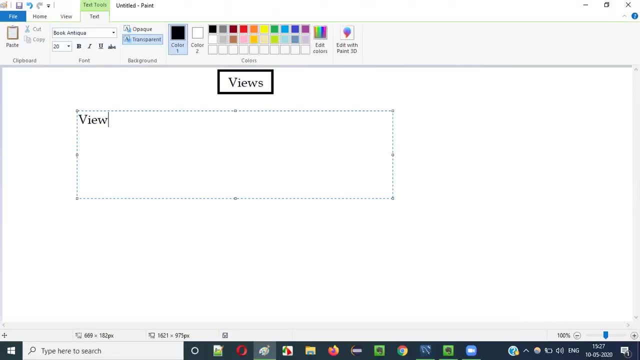 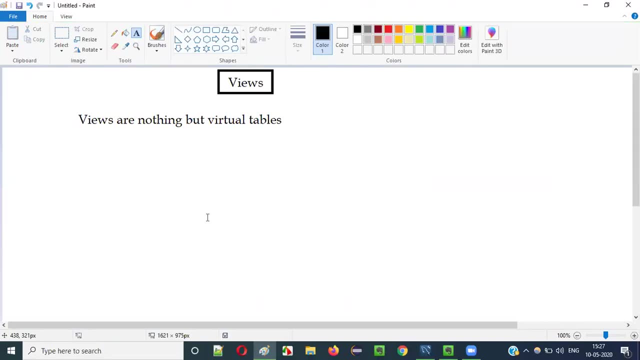 but the virtual tables Views are nothing but virtual tables, guys. They are not real tables, But they are created out of the real tables. Here we have real tables Instead of the need for creating a new table just because this table doesn't have. 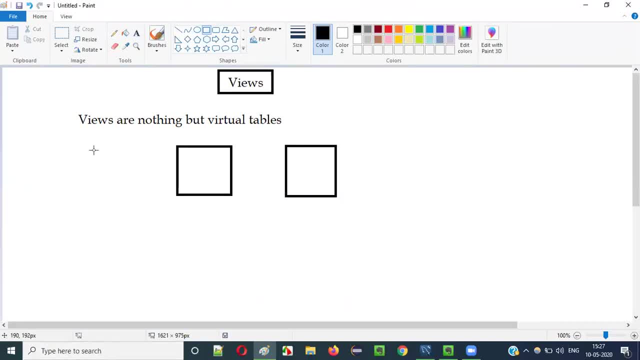 all the required things. So what we are going to do is we are going to create some virtual tables using the existing tables so that our requirement is satisfied. We don't have to create multiple tables or more tables necessarily. Instead of that, if we use 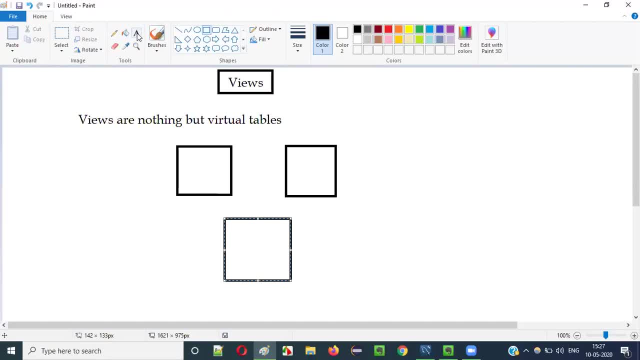 views. we can create virtual tables. This is a real table. Let's say this is a real table And you can create a virtual table based on your requirement in the application. So that is nothing but views. Now, one more advantage you get from the views is like: 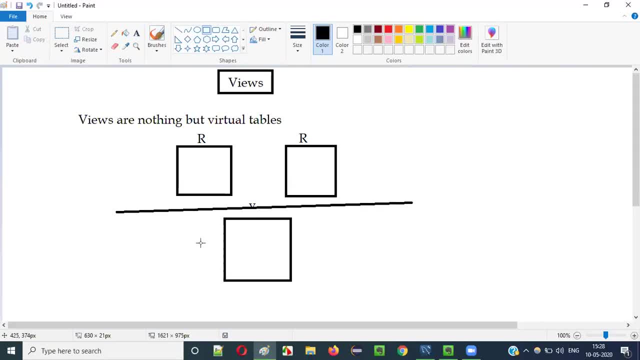 let's say, on a web page you went to an application web application in that there is some data displaying, There is some table data displaying like data is something like ID of the employees: employee name, employee salary, employee experience. All those details are getting displayed. 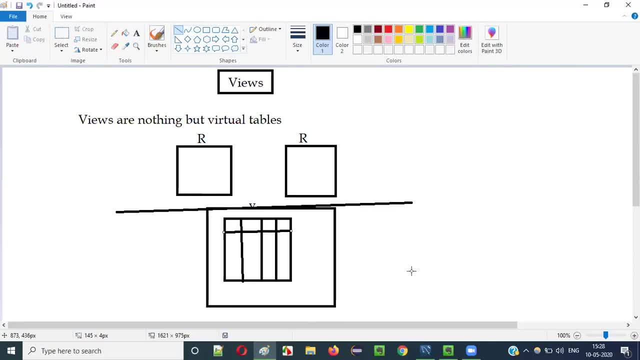 There is a page. So this person, who is actually viewing this particular table on the UI of the web page, doesn't know that at the back end there are two tables. He doesn't know that. this person doesn't know that all these columns are not from a single. 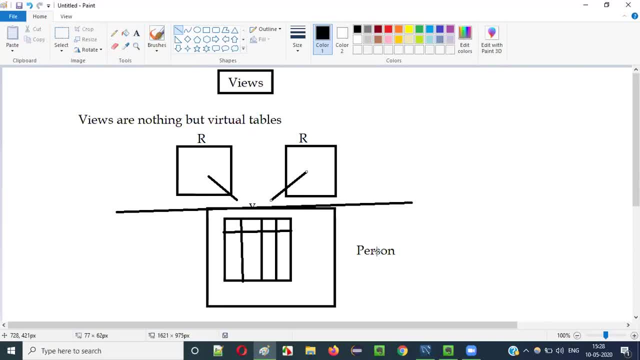 table. He doesn't know that There is a line of separation. This person don't know the internal working of the DB. In the DB, the database, there are two tables: Table 1, table 2.. From these two tables we can: 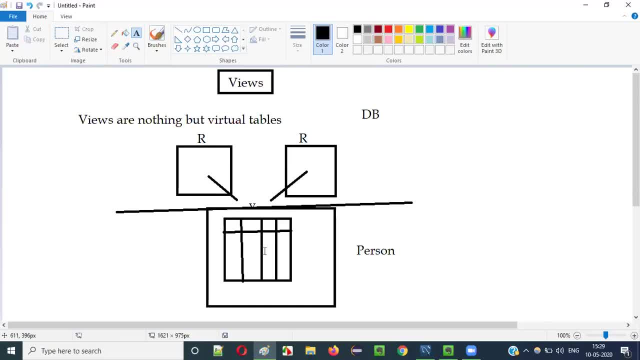 display on the web page. we can display in a single table all the required details for this particular person. This person will think that there is only one table inside, But internally there may be two tables, three tables, four tables, We don't know. But in the 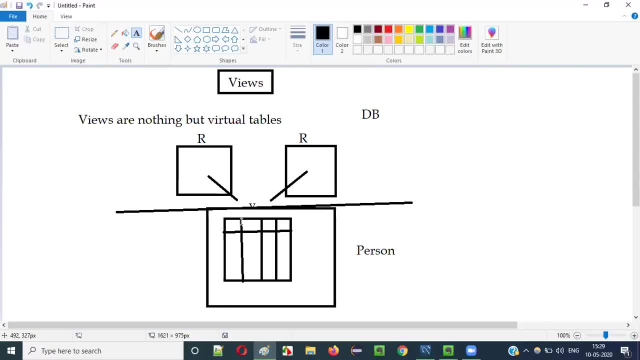 output, that is, on the UI of the application web page. it's being displayed as a single table. This is only possible with the help of views. We don't have to create tables for this kind of requirements. Today you may need four columns. Tomorrow you need five columns. Day after tomorrow you may need seven columns, or eight columns or nine columns, But every time for a small change, you don't have to create multiple tables. for six column table, seven column table, It is not required. Rather, what you can do is you can. 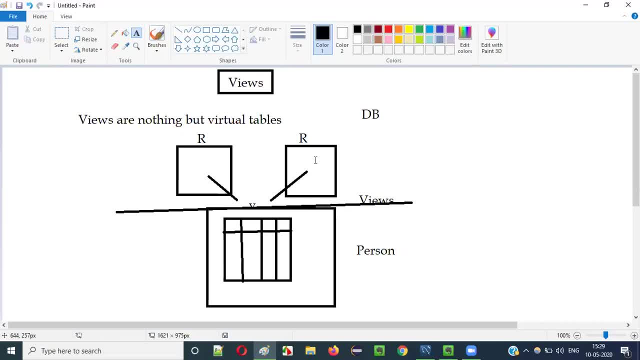 simply create views. That is, you can create the virtual tables using the existing table records, Then display it in whatever way this particular person wants. This is the main reason why we have to use views. We understand this concept. We understand this concept Practical. 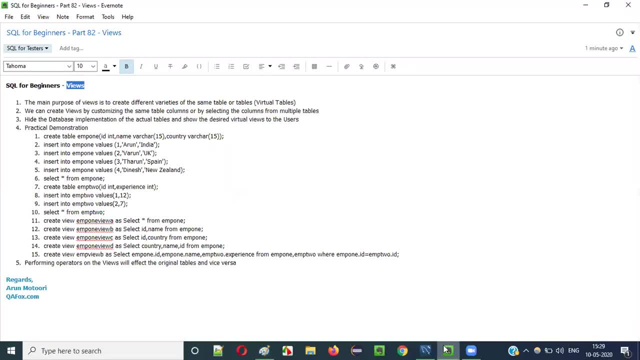 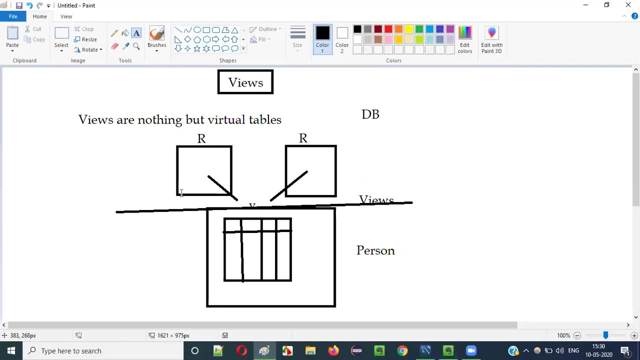 understanding will be very easy. Next thing is: let's go to the practical mode case. Whatever I explained so far, like creating views from a single table or creating the views from multiple tables, whatever it is- I am going to explain in a practical way now. 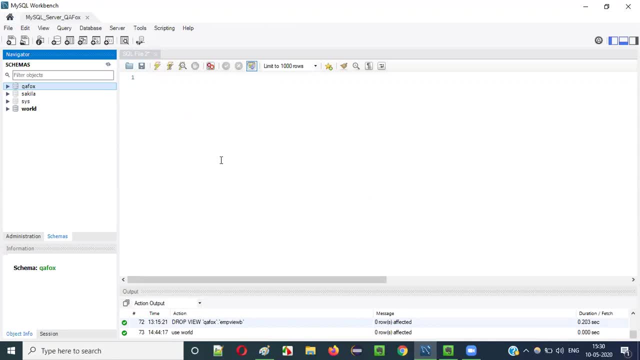 How to practically demonstrate is: I am going to use this database, QA Fox. Current selected database is world, But if I have to create some new tables or modify new tables or work with the tables under this particular QA Fox database, then I have to select this particular database. 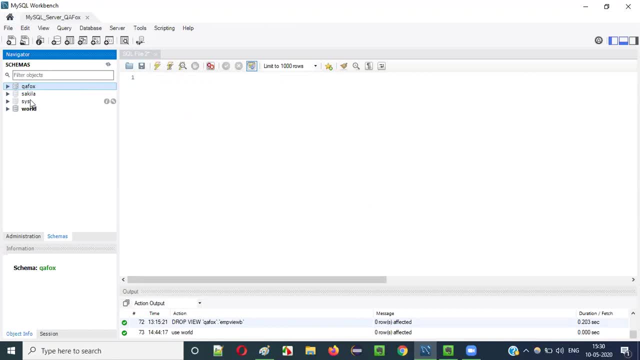 For your more information, there are four DBs here. These three DBs- circular sys and world databases- came by default in the MySQL. Coming to QA Fox, this is created by me in one of the previous videos. I am going to use the database. 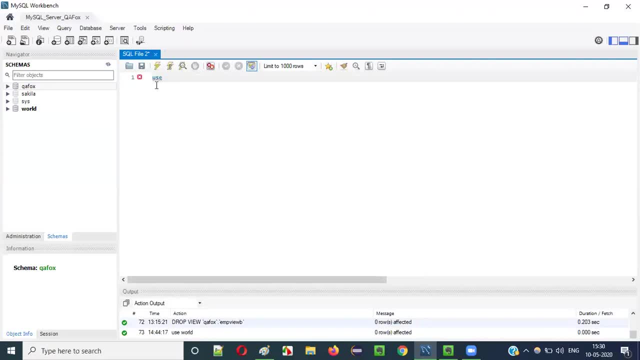 created by me. How to use that. I have to first select the database using this use QA Fox statement. When I run this, this QA Fox database will be selected. Once this QA Fox database is selected, what I am going to do is. 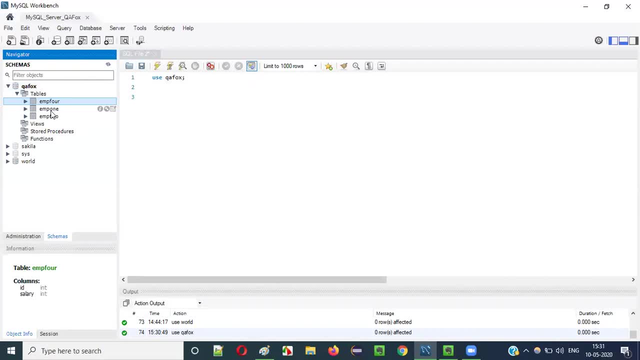 there are few tables which were created as part of the previous videos or whatever it is. Select everything and just delete them, Drop them. I don't want any tables to be there in this database. They got cleared it. There are no tables under this. 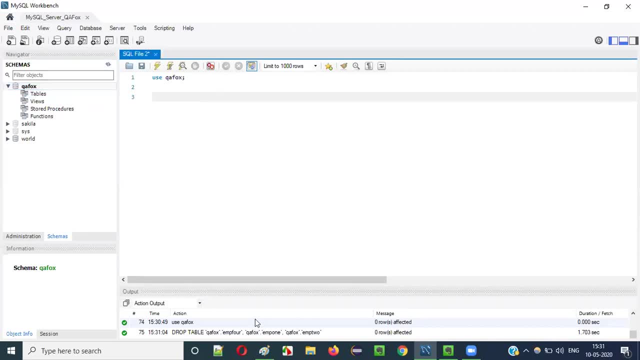 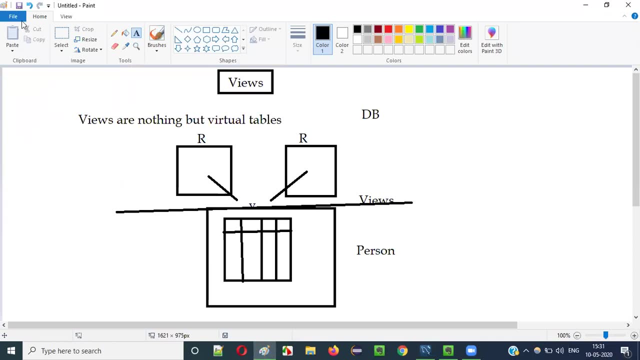 QA Fox database. I am going to create new databases. First database I am going to create is create table. I will show you what is happening in a diagrammatic format so that you can understand the things in a better way. Close it. It is not required. 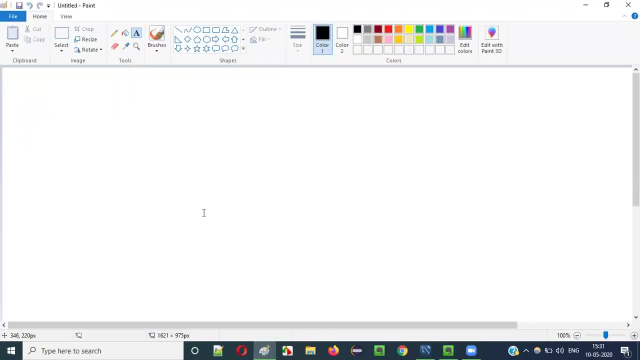 Whatever, I am going to practically demonstrate it. I am going to diagrammatically represent it at the same time. First, what I am going to do is I am going to create a table. The table is EMP1 table, EMP1 table. 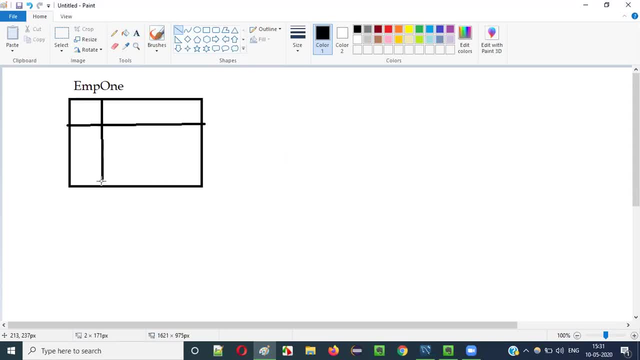 It will be like this: It is going to have three columns. EMP1 table is going to have three columns. The first column is ID column- ID of the employee. Then second column is going to have the name. Third column is going to have 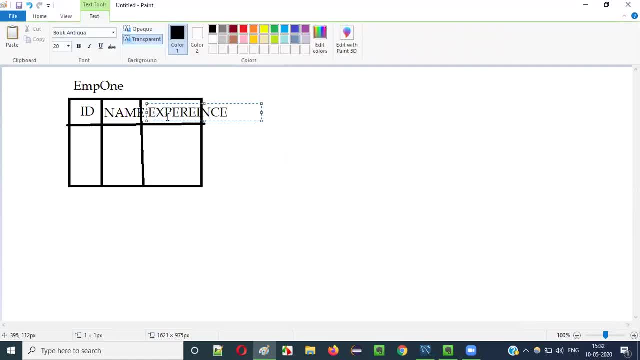 the experience. Third column is going to have the experience. Fine In this, some four records I am going to insert In this. I am going to insert some four records. I need another extra record here, Four records. I said This is extra record This table has. 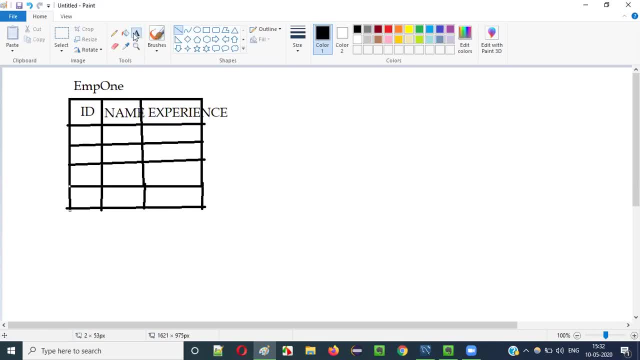 four records: One, two, three, four. In the first record I am going to give one record, Then this one, Faroon experienced as twelve. Second one is a two. Then Varoon experienced as seven, Then three Tarun. 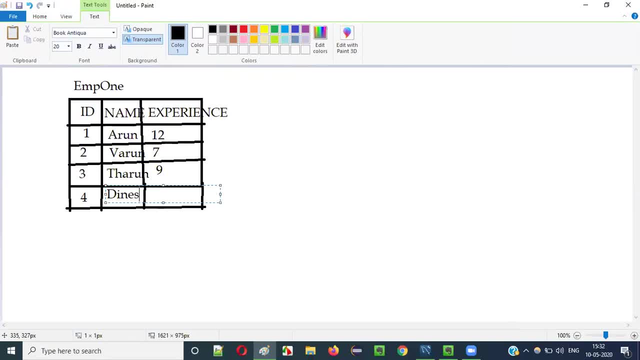 experienced as nine. The fourth one, Dinesh, experienced, as is this emp1 table that i am going to create. practically, i have to create the data right. we not to explain views. i have to set up this kind of tables. then only i can explain. 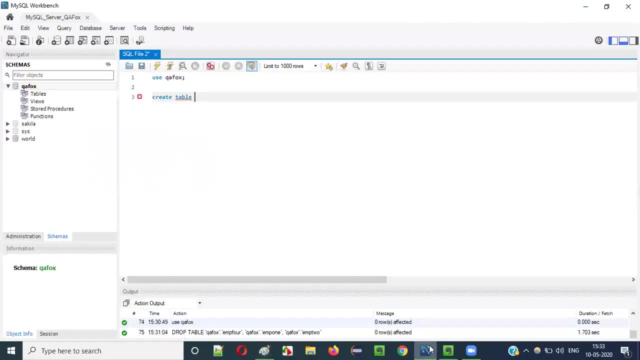 so let me, let me create this table and based on that, i can explain views later point of time. so create table. what is the table guys? emp1 table, okay, emp1 table. the records are like, the columns are id as in name, as worker and uh, the experience has uh, inter. okay, like this, i created a table, so i have to run this first, okay, 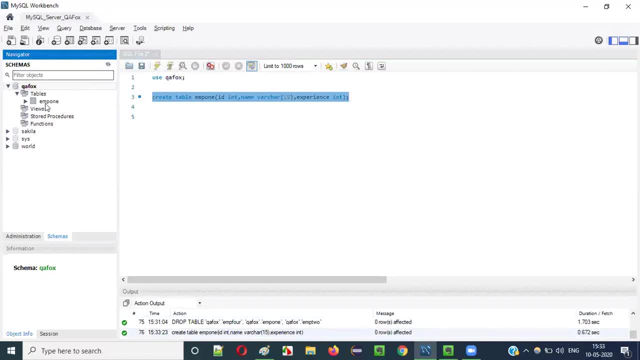 then only the table will be created. so once the table got created- refresh here you can see the table here- emp1 table got created and, uh, whatever the columns i mentioned, those will be there under the columns you can see here. id name, experience are the columns in this emp1 table. now, after that: 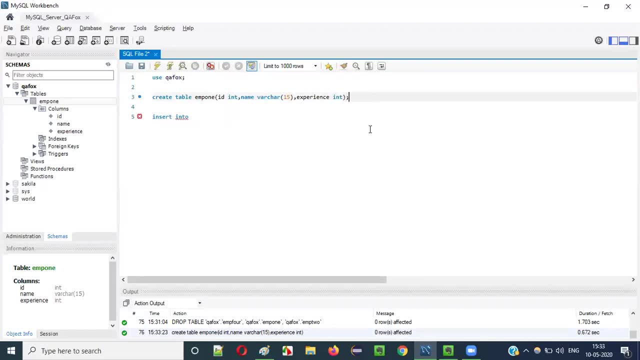 i am going to insert some records into this table. by default, when you create a table, you will not see any columns, i mean you will not see any records. if you say select star from emp1, empty table will be displayed with the only the column names. okay, 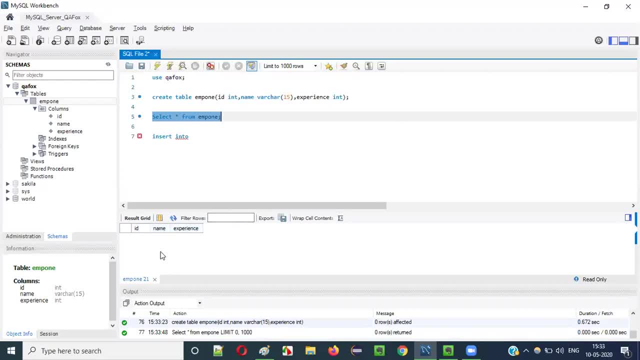 without any records. you see id name experience columns are there without any records. now i have to insert some records into this table. how to do that? insert into emp1 values as values as one comma, same records. i am going to insert guys: one around, two around seven, three around nine and. 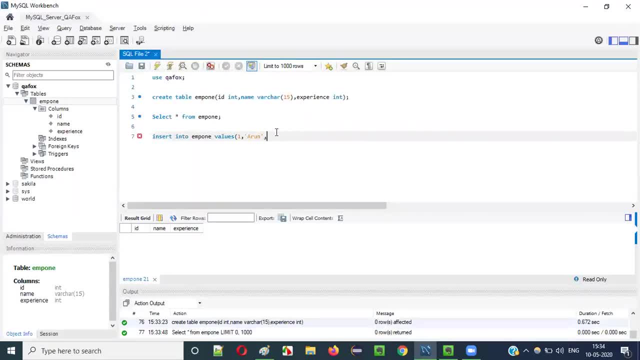 four finish eleven. okay, one around twelve. insert into emp1 values as two varun experience as seven. insert into emp1 values three comma around experience as nine. insert into emp1 values four comma finish experience as 11.. like this, i i will insert four records into the table. 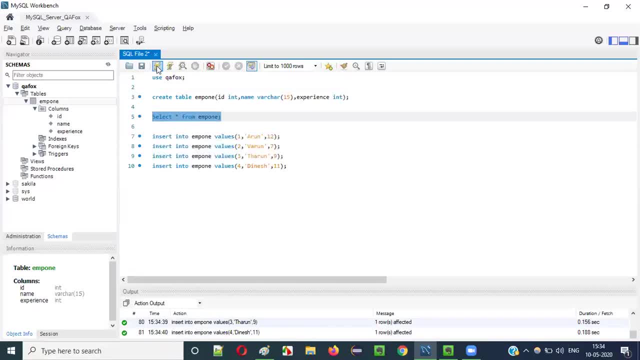 so after inserting these records, let me say select star from em1. You see, all these four records got inserted into the table. Now we have a table. So on the top of this table I am going to apply views. How to create views. There is a requirement. 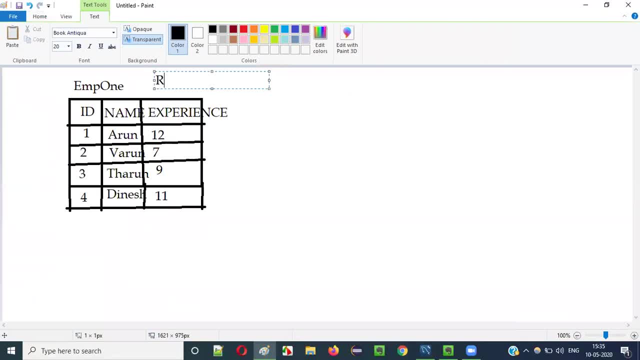 Let's say this is a real table. But tomorrow a requirement came where I need to create a table. I need to create a table which has only ID and name. Only a table need to be there which should have ID and name guys. Only ID and name should be there. That is the requirement. 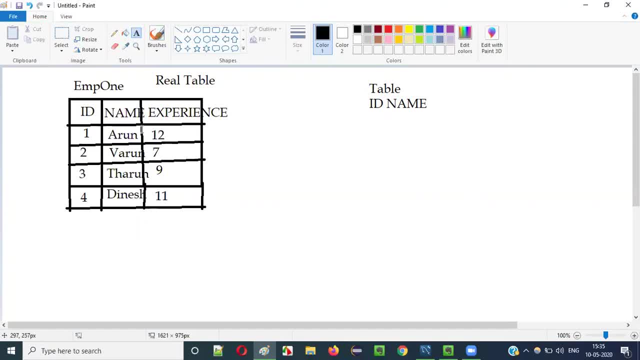 For that I don't have to create another table. Rather, I can create a view for the same existing table And use it as another table and display it to the people. That is better right, Rather than creating multiple tables just for the small sake of the requirement changes. 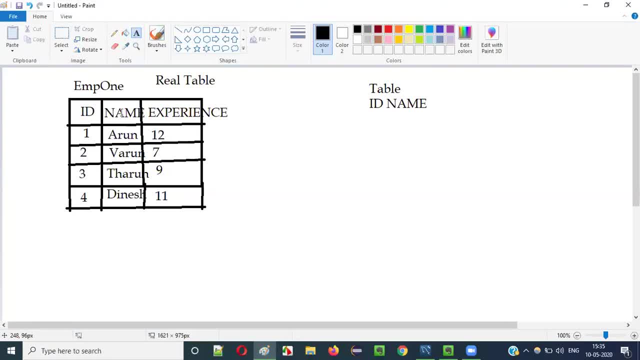 So what I am going to do is I am going to create a view which will only contain this, Based on this EMT1 table. I am going to create a view Which will only contain this, Which is nothing. View means what, guys? 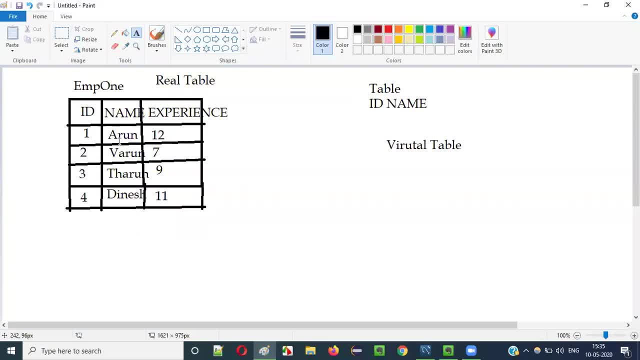 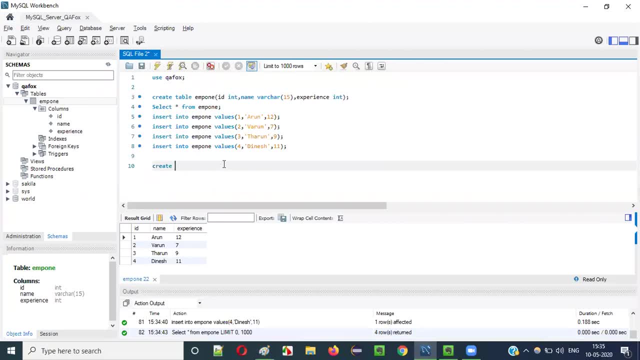 Virtual table. Instead of creating a real table, I am going to create a virtual table Based on the existing tables, Based on the changes requirements. That table is going to have only ID and name. How to do that? Create View. 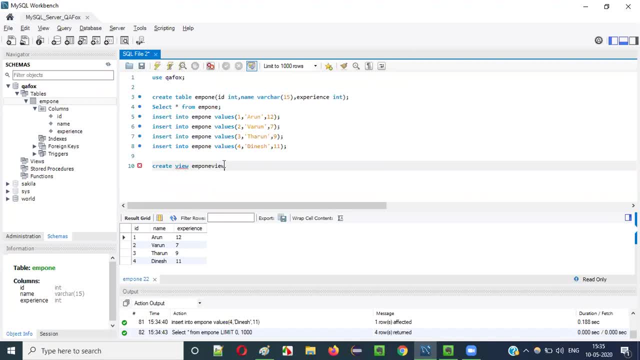 I have to give the view name, guys. What is the view name? EMT1 view. Okay, EMT1 view, So Create view EMT1 view, As I have to use as Select Star From. 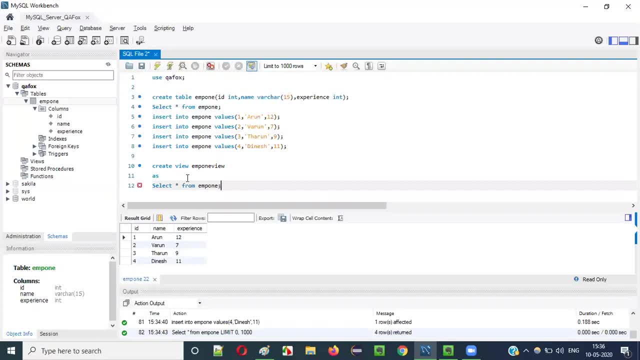 EMT1.. What will happen if I do so? All the columns from the EMT1 table will come into the EMT view. Okay, I don't want all the columns. My requirement is to only have the ID and name, Not experience. 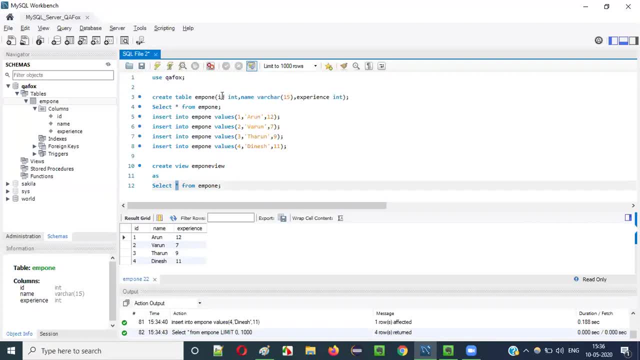 So instead of the asterisk symbol here, I will say ID comma name. Now, What I am going to do is: This is a. This is enough, guys. Create view, The view name, The view Virtual table or view that you are going to create. 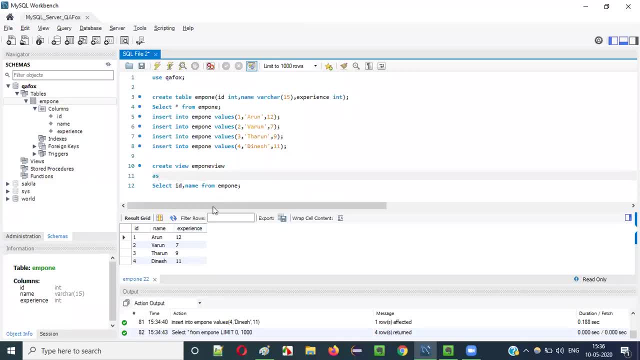 Its name is going to be Emt1.. So What I am going to do is This is a. This is enough. guys, Create view, The view name, The view Virtual table or view that you are going to create. 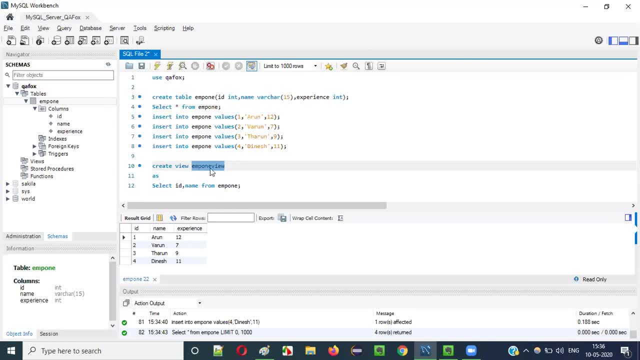 Its name is going to be EMT1 view Okay, Which is Being created on the based of EMT1.. Okay, I have to say Create view View name As Select, Whatever the columns that are needed for that particular temporary table. 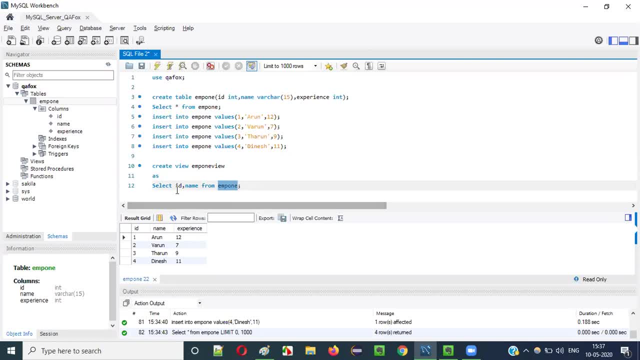 I mean Not temporary Virtual table or Okay, View ID, comma name From Original table. That is A real table, EMT1.. You have to say Now, If I run this, A view will be created. 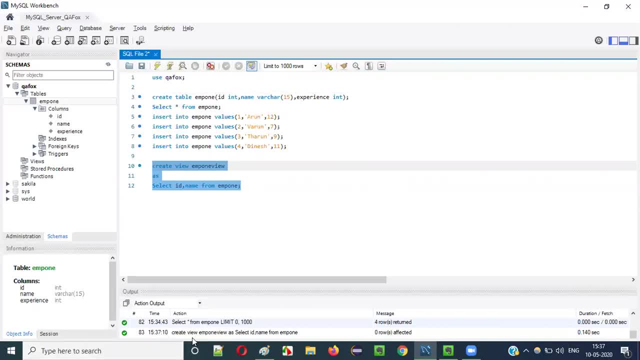 Okay, A view. So Create View Got Successfully Executed Here. Now How to find? So How to find The records That are there in this particular EMT1 view. Similar guys, Same thing. 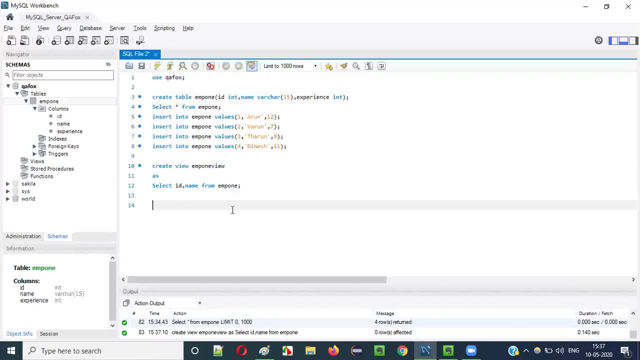 Same statement You have to use Here: Select star from Real table name. Here You will say Select star from View name. If you say Select Star From View name is You will get All the records. 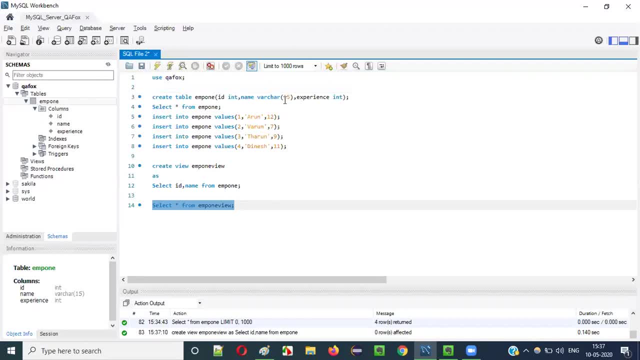 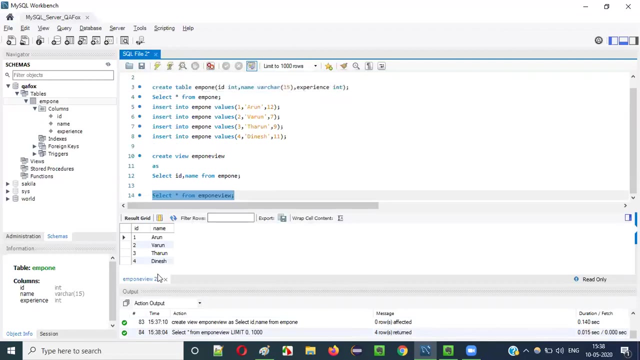 That are actually There in the EMT1.. But only from this ID and Name column, Because Here I clearly specified: Create View EMT1.. View As Select: ID, Comma Name. 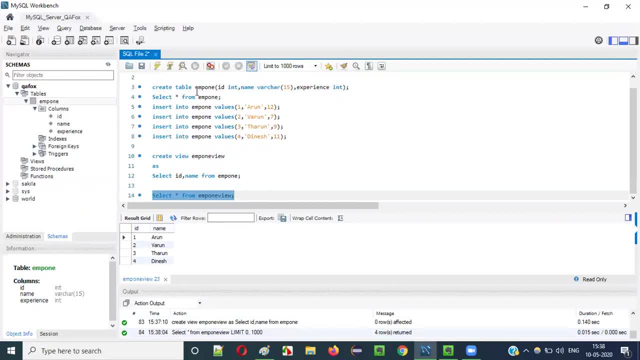 From EMT1.. Only ID And Name Will be Coming From There. Only ID And Name Should Be There. For That Reason I Don't Want To. 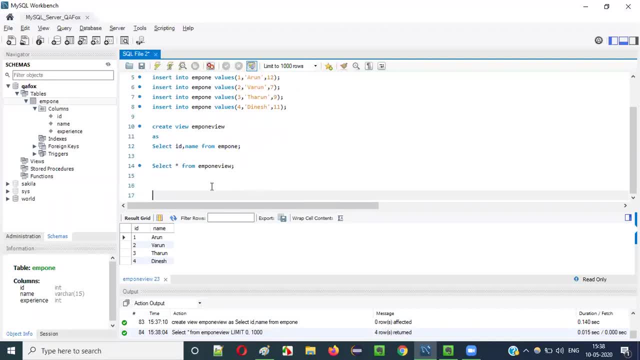 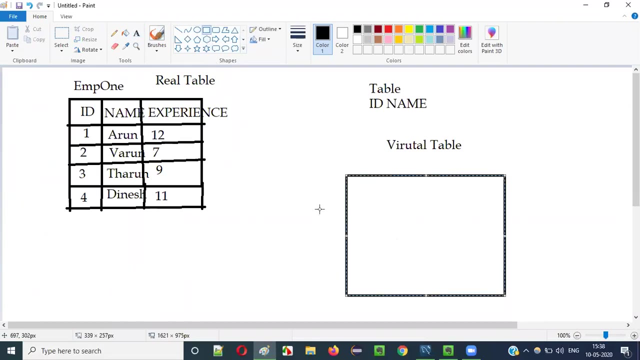 Create Another Table. Rather, What I Will Do Is Using The Existing Table. I Want To Have A Table To Be Displayed. That Table Should. 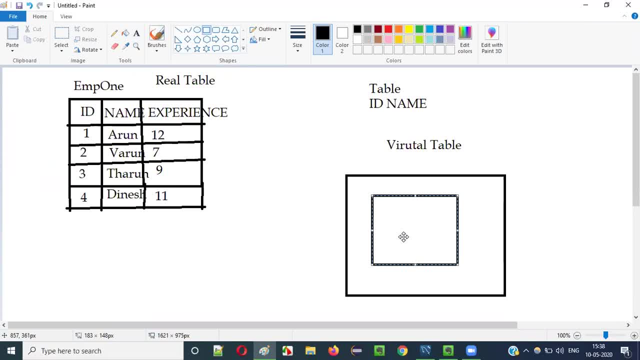 Have The Employee Details. Okay, The Same Employee Details Are Required To Be Displayed On This Table, But All Is Displayed On This Particular. 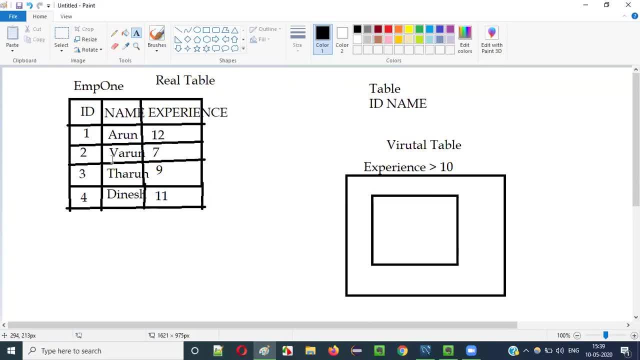 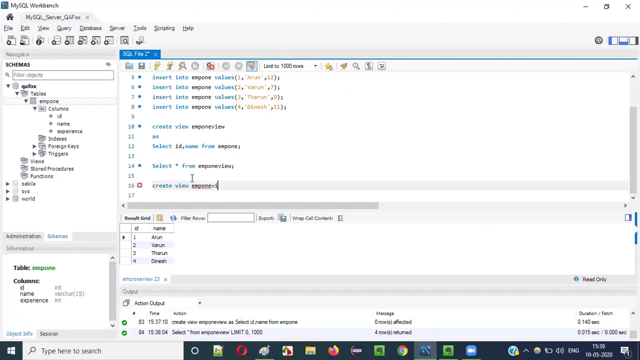 Table Of This Webpage. Again, Do I Have To Create Another Table? Right, I Don't Have To Create Another Table. Even You Can Simply Create. 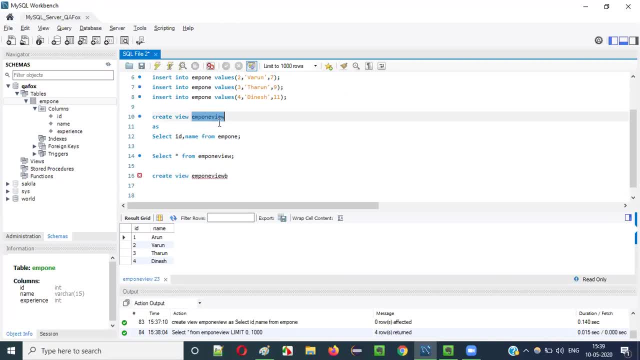 Another Table Of View, One View B. So Just To Differentiate With This EMP1. View I'm Just Giving Employee. EMP1. Something B Letter I'm. 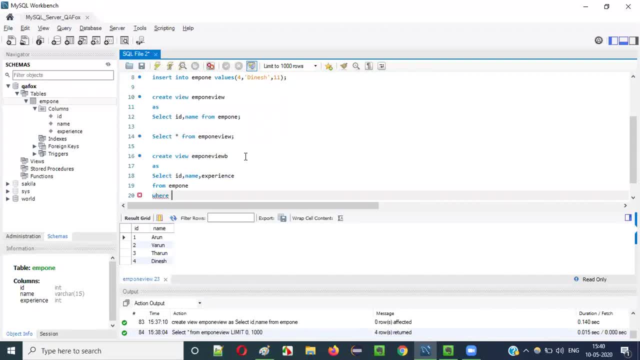 Adding So That This View Like This Also. Okay, So, Where Experience Is Greater Than 10.. So, Whatever The Table That Is Going To Be, 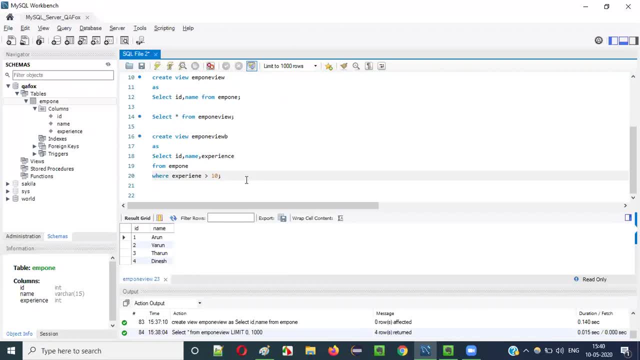 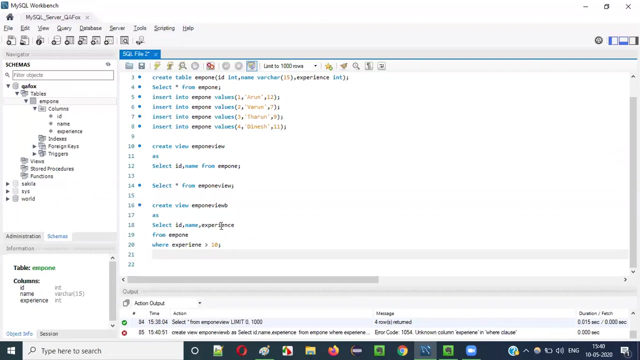 Virtual Table That Is Going To Be Created, Based On The Experience Of The Employees Whose Experience Is Greater Than 10.. This Is A Better. 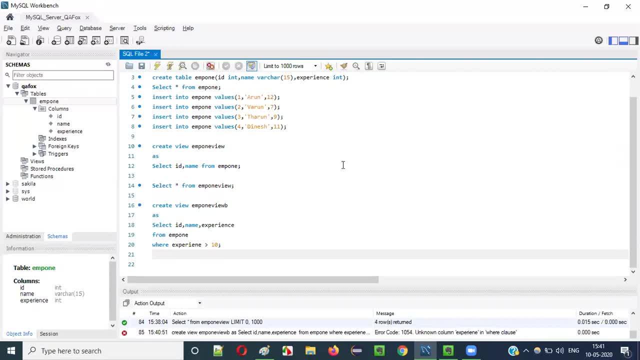 Way. Instead Of Creating The Table, We Have To Do Like This. Okay, Let Me Run Again. Now. The View Got Created. New View With The. 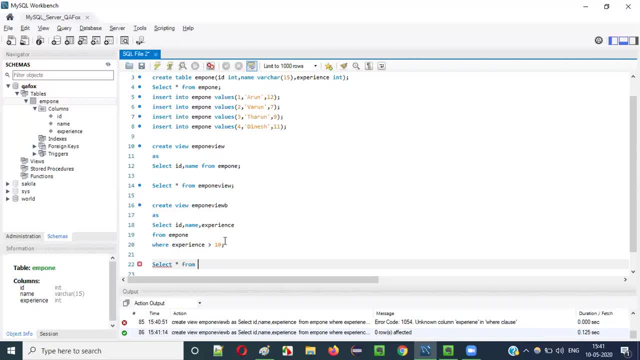 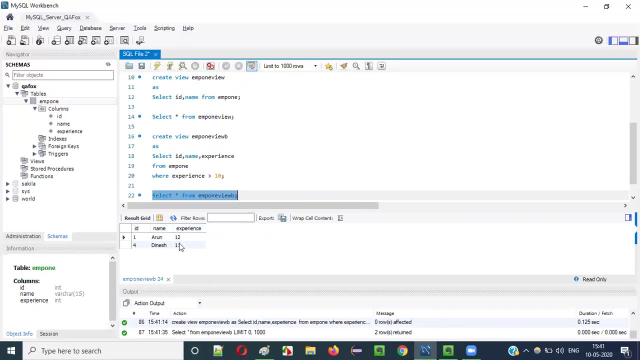 Name: EMP1.. View B Got Created, So How To Find The Details In That Particular Table? Only Two Records Are There. Having Experience Greater Than 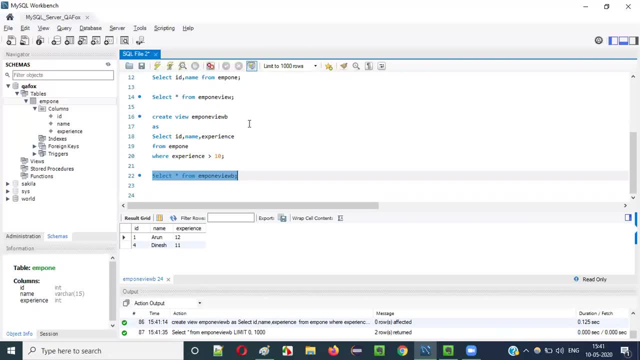 10. Okay, Greater Than 10.. So In Real Time We Make It Different Type Of Requirements Where We Need To Create A Table In One. 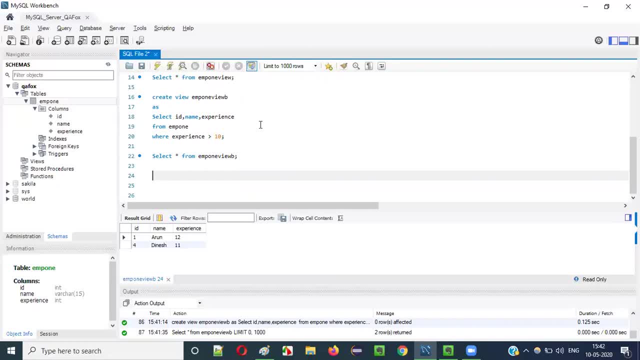 Case Where You Don't Need All The Four Columns. Only Three Columns Are Required. In Another Case There Was Requirement Where The Experience Of Let's 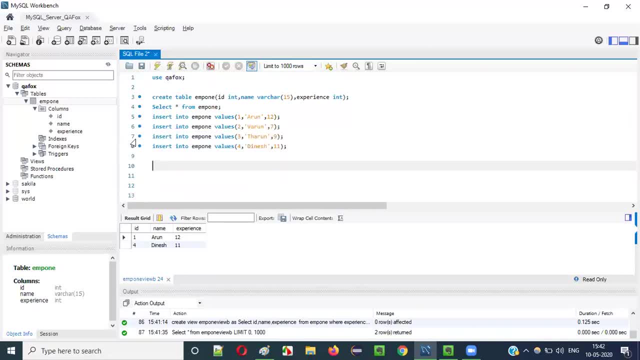 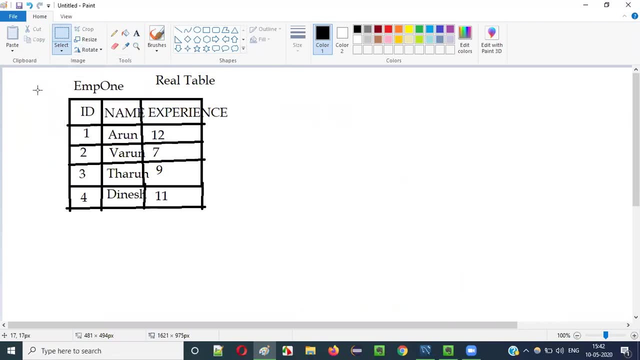 Say There's Another Requirement Where, Okay, There Are Two Tables, Okay, Here, Only One Table Is There. But There May Be Some Other Cases Where 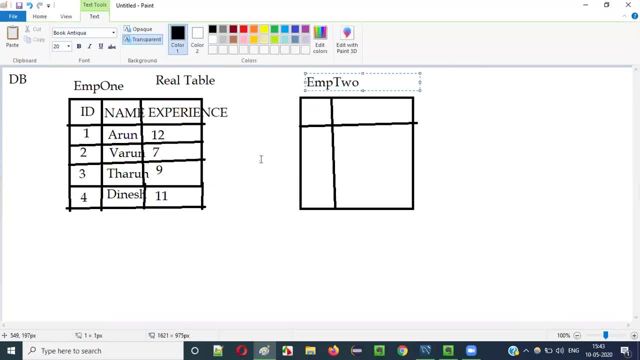 In The Database. This Is Also A Real Table. One More Real Table Is There. That Is EMP Two. Okay, Here Real Table Is EMP One. 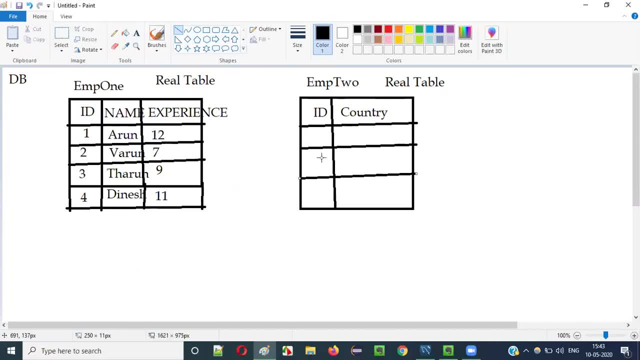 Here Also Another Real Table. That Is There. Three Is There. Okay, So Here Country, I Am Saying India, USA And UK, Okay, Fourth Record Is: 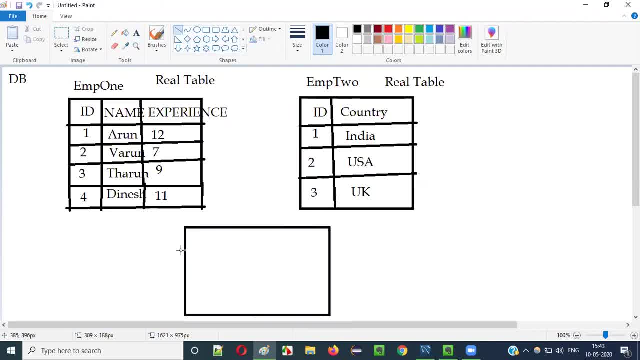 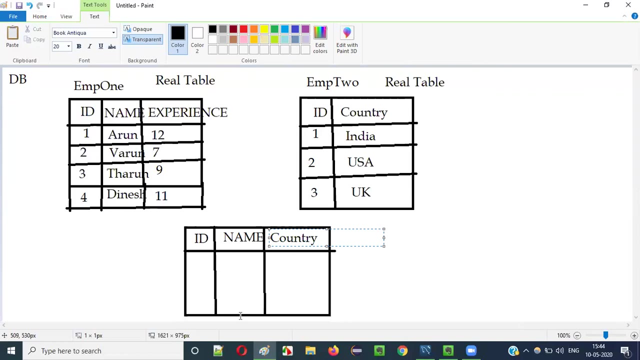 Not There Here, Only In The EMP One Four Records. These Details Should Be Displayed. That Is I D Name And Country, So Here Name. 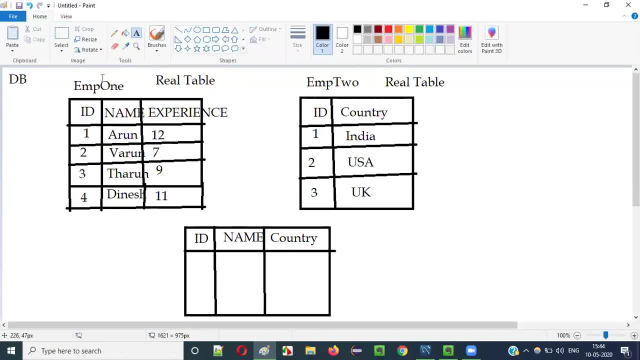 Is From One Column. I Mean I, D And Name Are From This EMP Two Table. Does It Have The Name? But Country Is Belonging? 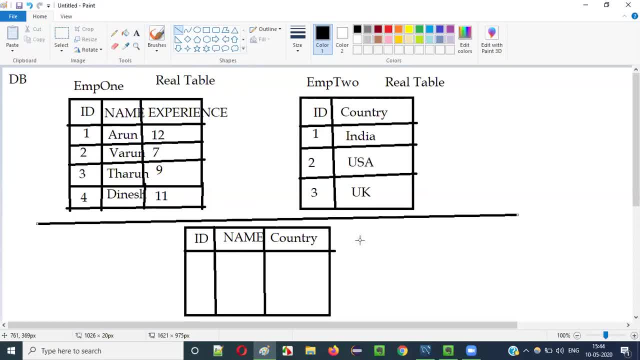 To The EMP Two, Which Is Not There In The EMP One, But The Resultant Table. That Is A Table. So What We Have To. 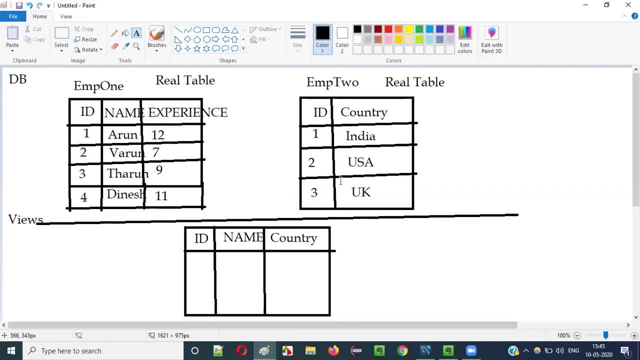 Do We Have To Create Virtual Tables Using Views? Okay, We Have To Apply Use Where, With The Help Of Use. We Have To Do This. 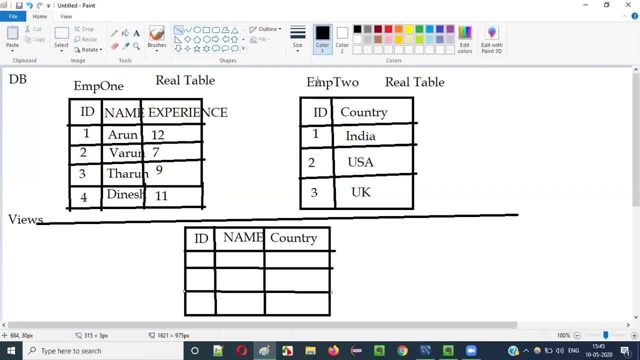 Okay, So What I'm Going To Do Is I'm Going To Compare If The Idea Of This Employee One Is Equal To The Idea Of 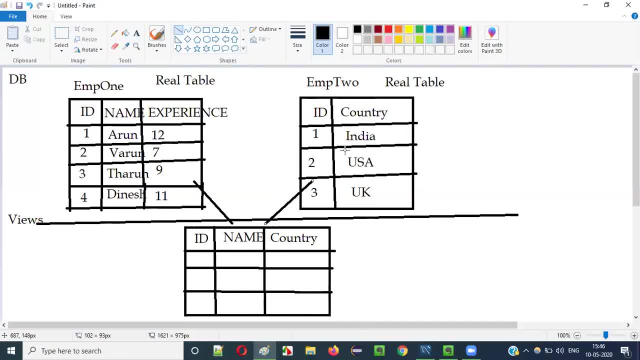 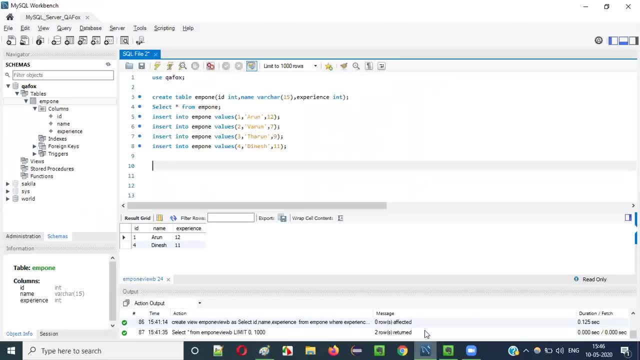 This Table. Okay, So Let Me Practically Show You How To Do That. Before, Before Creating A View, We Have To Create This EMP2. Table. 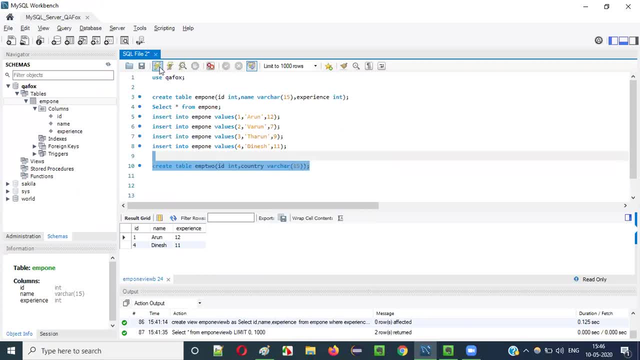 We Have Already Have Started With EMP2.. Name By Default: It Will Be An Empty Table Guys, If You Say Select Star From EMP2.. What? 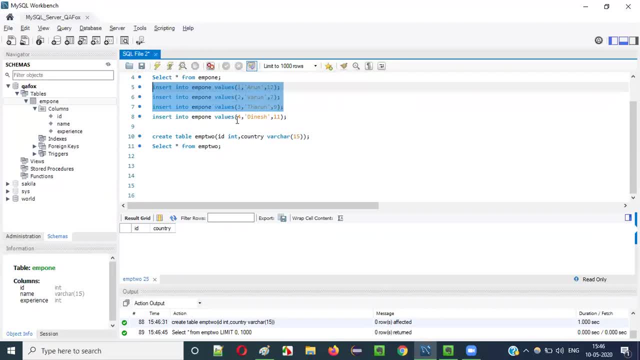 Will Happen. Empty Table Will Be Displayed With Values As One Comma Country. I Am Giving India Okay, So Then Insert Into EMP2. Table. 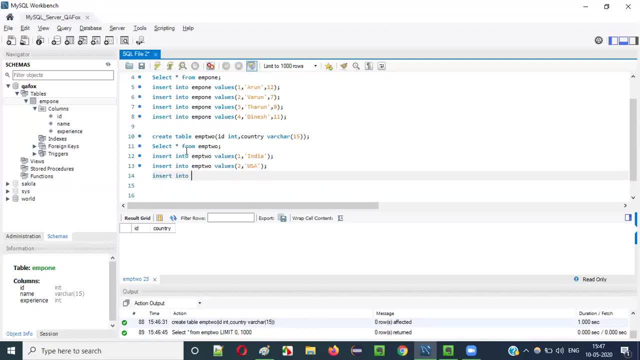 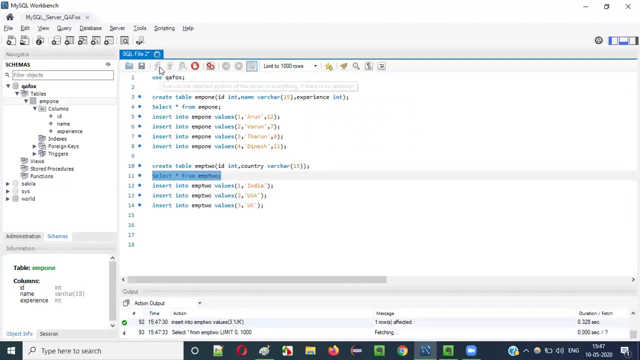 Values As Two Comma USA, Then Insert Into EMP. To Values As Three Comma, Set A Ones. Okay, All The Records Will Be Inserted. 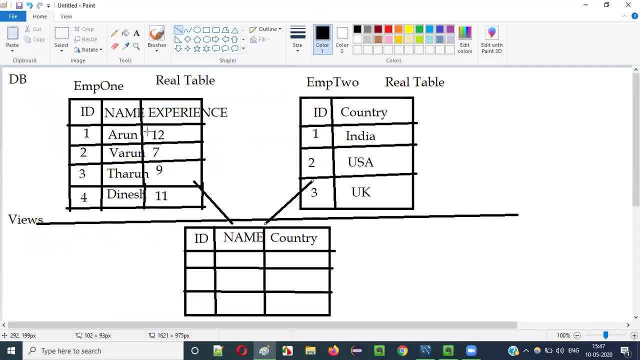 Now Select Star From EMP2.. This Time You'll Get Three Records Inserted Into This ID: Country Columns Of This Table. Okay, And Create The. 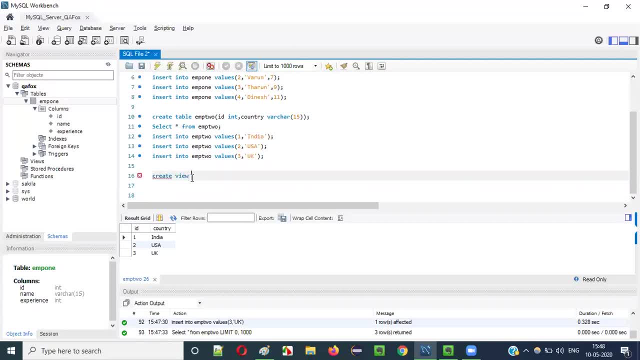 Resultant Table. How To Do That? I Have To Say: Create View, Create View, EMP View. Okay, I'm Simply Giving EMP View As Here To: 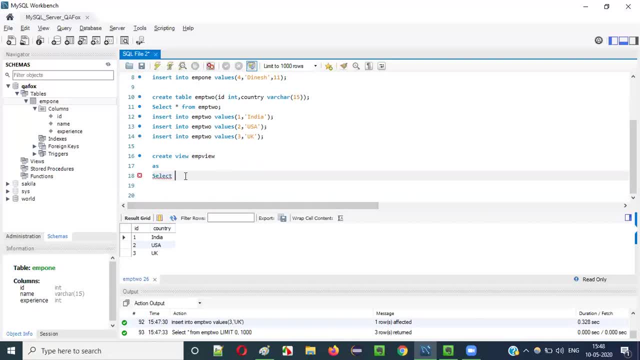 Get The Records From The Two Tables Okay. In The Single Result We Can Use Select Statements Right. Select What Is Required ID Is Required Name. 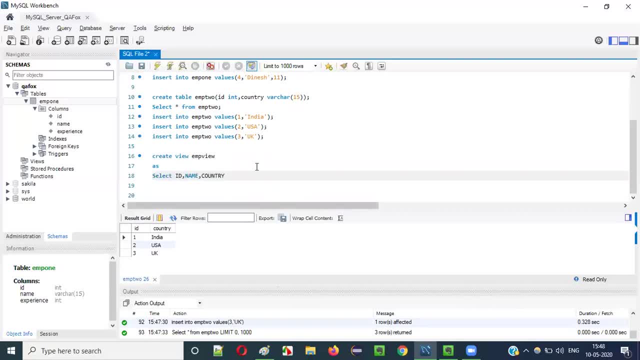 Is Required. So To Overcome That I Have To Give The Table Name Here From EMP One, EMP Two Tables. Okay, So Here I'm Specifying. 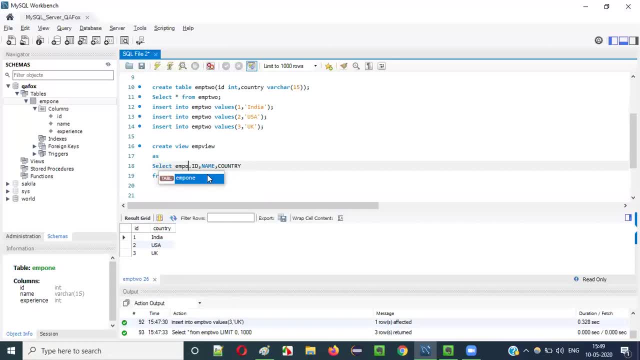 EMP One, EMP Two, Tables Two. So From One Table This ID, Because This ID Is There In Both Tables. Better To Give One Table As 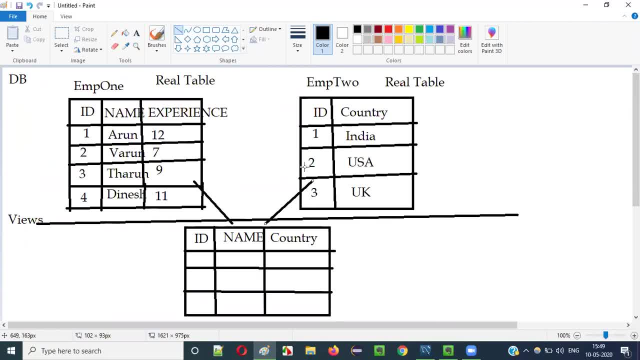 Reference. And Here I'm Going To Add A Condition For This Particular Table: Only One, Two, Three Records- India, USA, UK- Will Be Displayed. 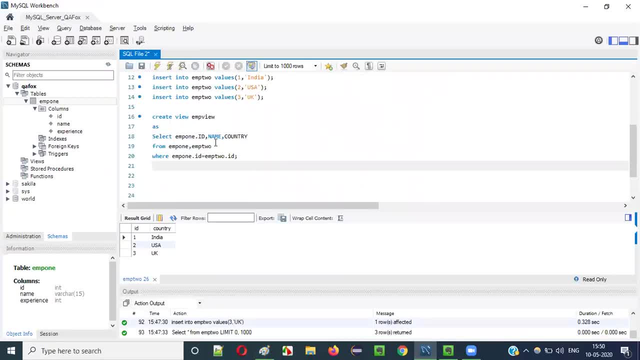 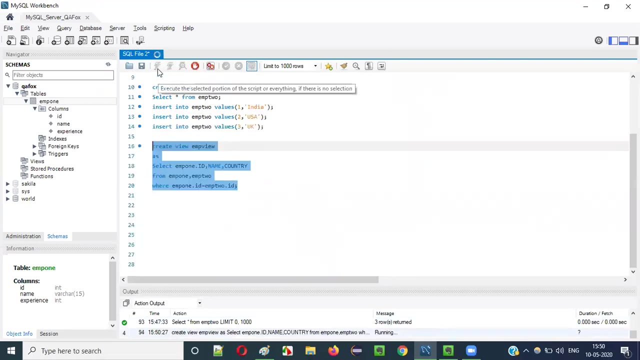 Okay, But For Dinesh Nothing Is There Here, So It Will Be Ignored. So Run This Now. So The View Got Created With The 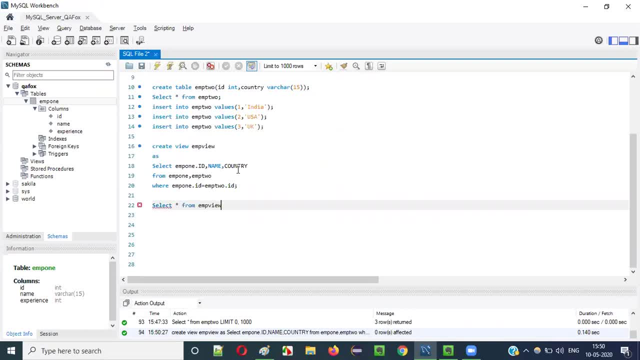 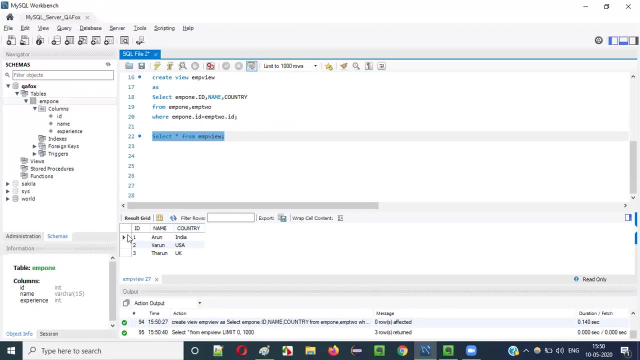 Name: EMP View. So We Have To Find Out What Is There In That EMP View. Select Star From One To Three, Around Around India, USA. 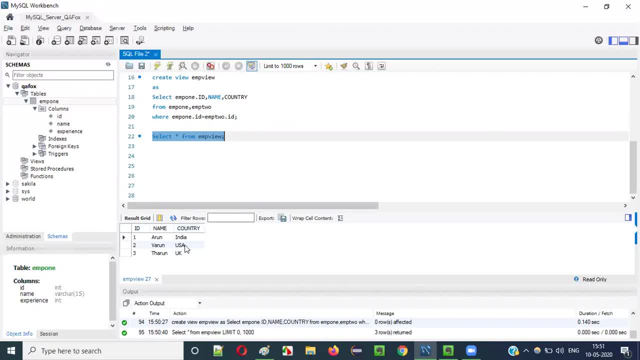 UK. Whatever The Result, We Want This Table. Now I'm Going To Show On The Web Page Of The Application Instead Of The Two Columns. 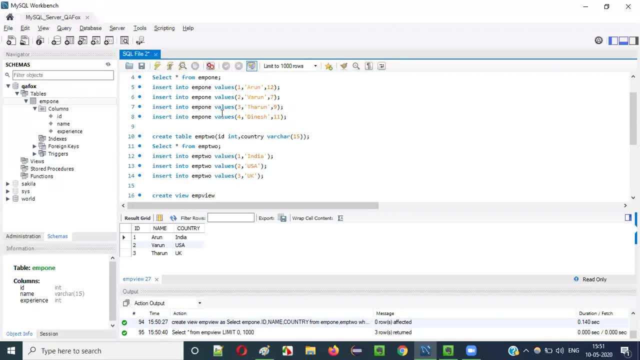 Out Of That Single Table Okay, Whereas Complex Views Are Where You Have Multiple Tables And You Have To Create Another Table Out Of That Existing. 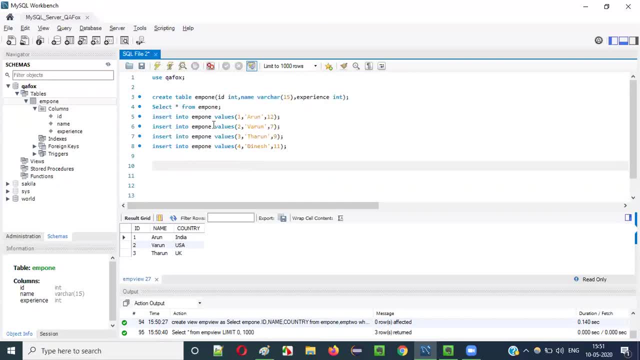 One Table For That Particular Understanding Of That. What I Mean To Say Here Is, If I Create A View Based On This Particular Table, 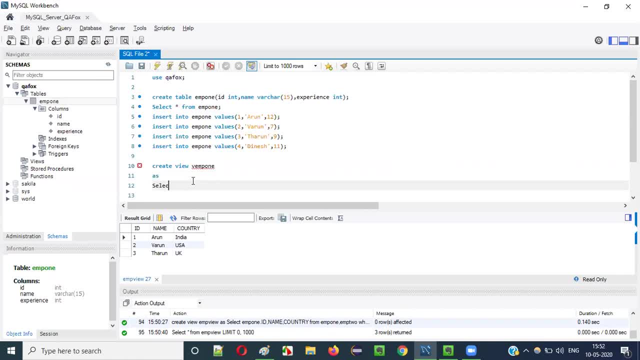 Let's Say, I Create A View Based On This Table. Okay, So What Will Happen? So What Will Happen If I Say Create View? 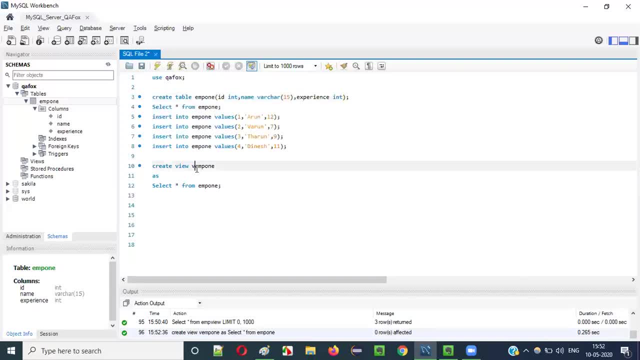 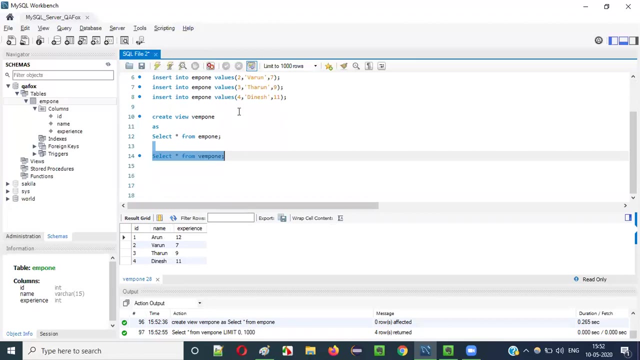 V- Emp1.. As So, Based On This Emp1.. Table V- Emp1.. View Is A View. Right Is Not Emp1.. It's A View- Emp1.. 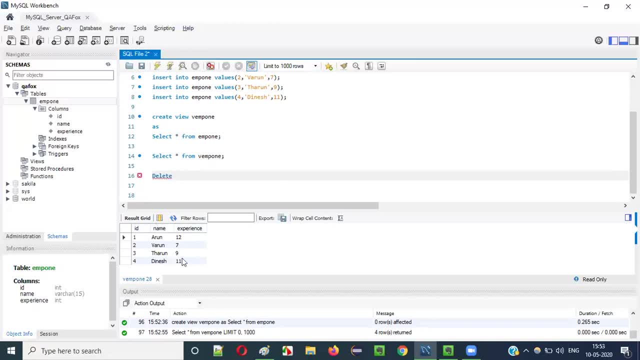 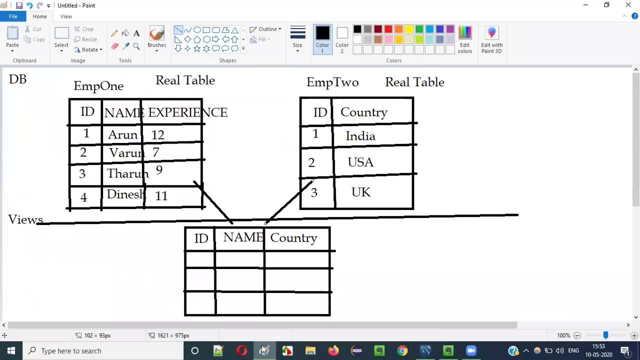 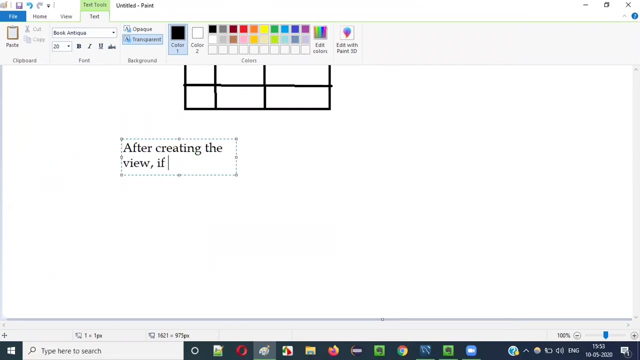 Okay, So Run This, The Replica Of That Original Real Table, As Form Of The View. If I Insert Any Records Into The Real Table, Okay, 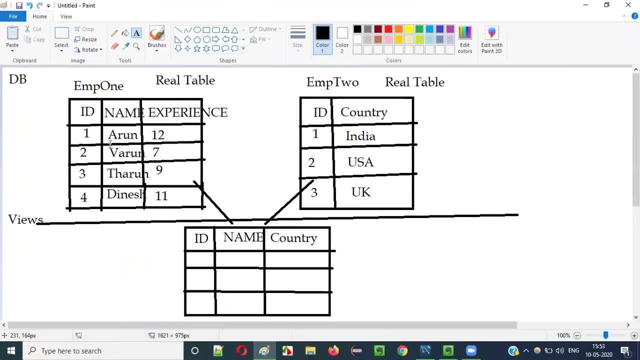 On Which, On Which We Have Created The View. What Will Happen? You Are Understanding Right. This Is The Real Table. There Are Four Records. 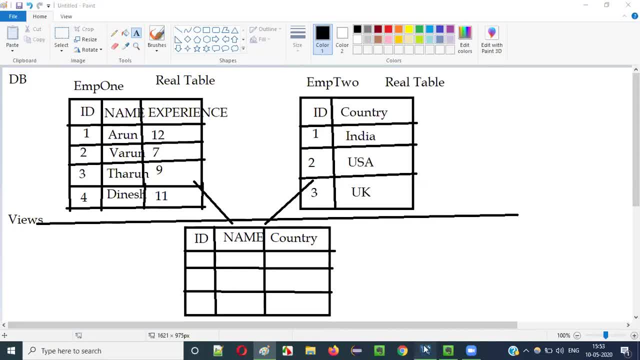 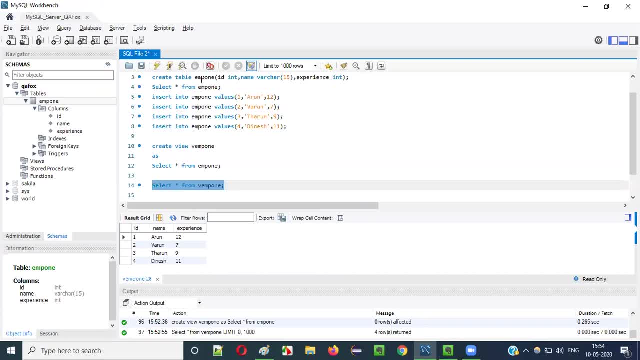 But After Creating The View Here, I Inserted One More Records. If The Record Okay, Then What Will Happen To The View In Iran? Okay, 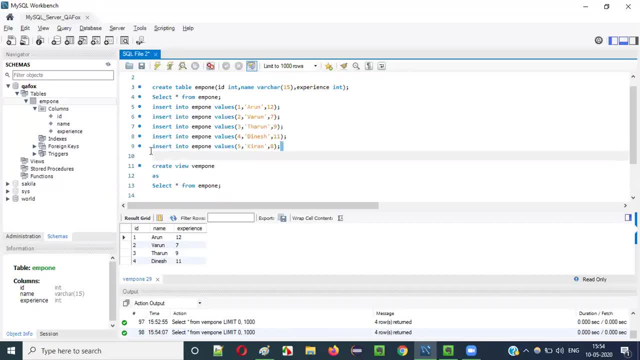 Iran, And I Will Say It Like This: I'm Trying To Insert One More Records, If The Record, Into The Mp1. Table. So If I